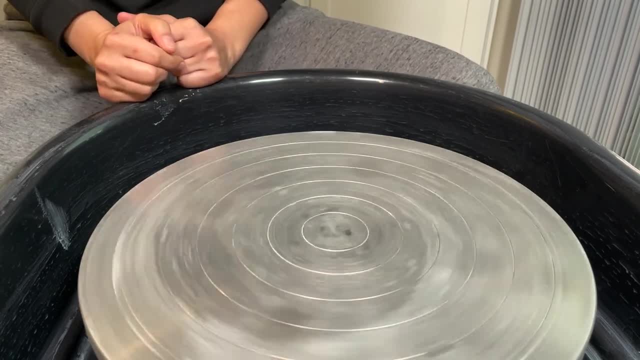 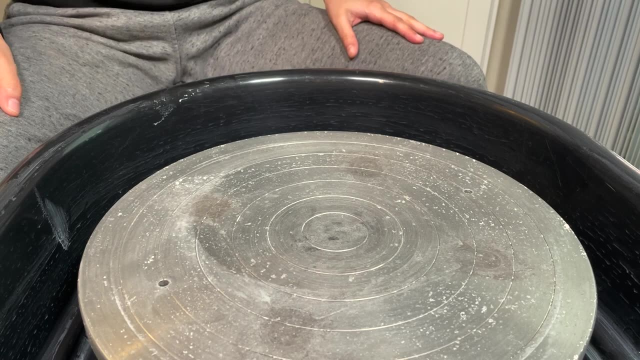 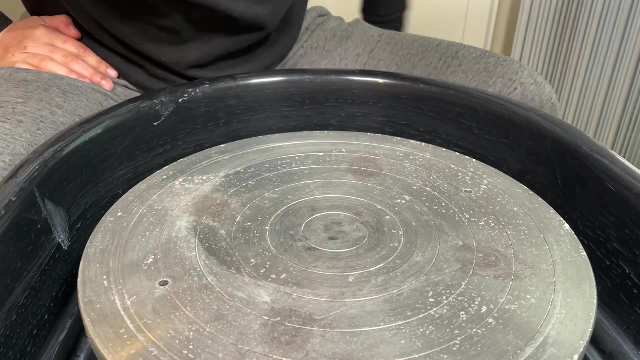 release my foot and it will maintain that speed. I'm going to press down on my heel again to get that off. In terms of our setup, you want your feet to be level and your nose to be above the wheel head and over the center. Especially as a beginner, you're going to want to be able to lean. 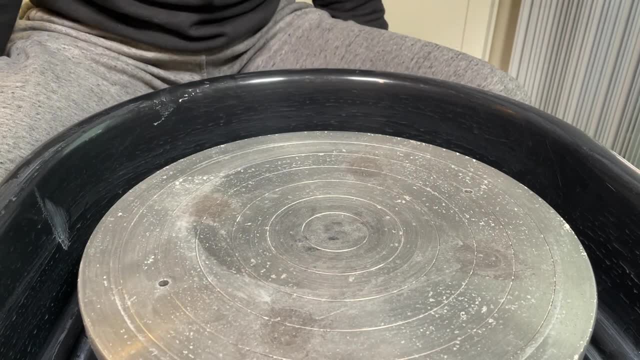 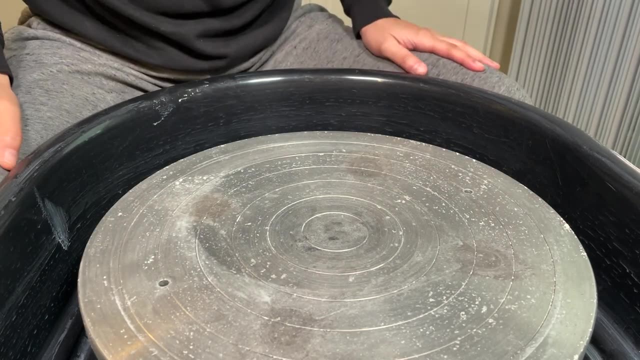 on each leg for support, So make sure to put support under your leg. Usually, most studios will have bricks. I use yoga blocks just because that's what I have around. In terms of the direction and where we focus on the wheel, I'm going to put my foot on the wheel. I'm going to 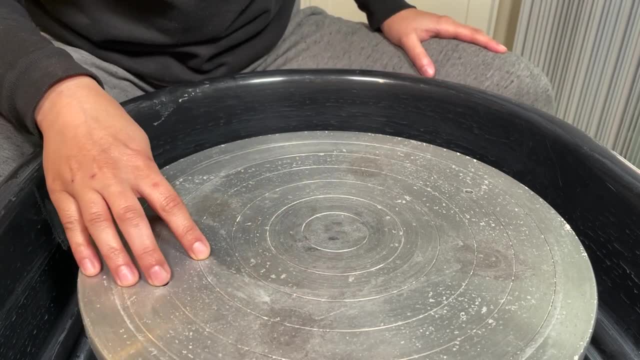 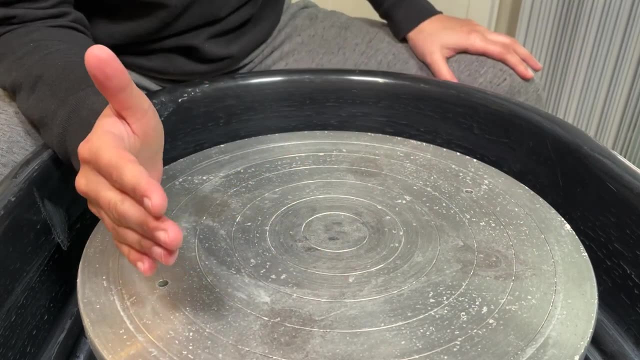 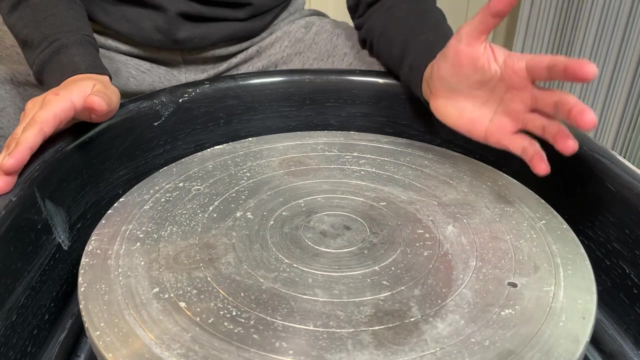 put my foot on the wheel. If you're right-handed, this is the sweet spot, and you're going to want the wheel to turn into your palm. If you feel it turning into your fingertips, that is the wrong direction. So you can flip the direction of your wheel using a switch. And if you're left-handed, 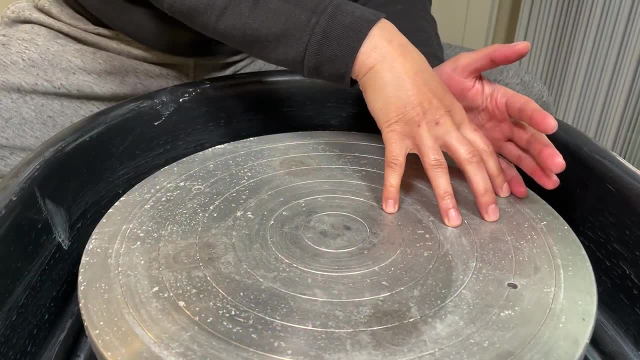 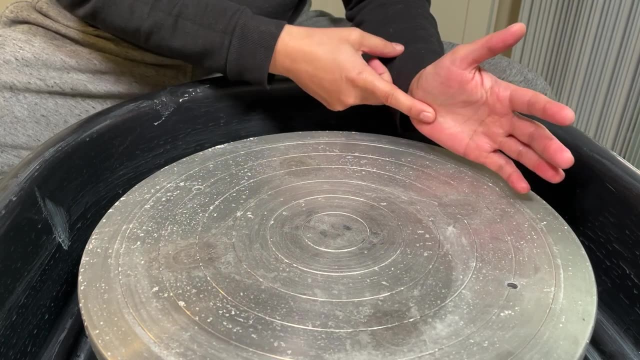 you're going to want the wheel turning into your palm. This side will be the sweet spot, the left side of the wheel, And, again, if you feel it going into your fingertips rather than your palm, you're going to flip the direction. 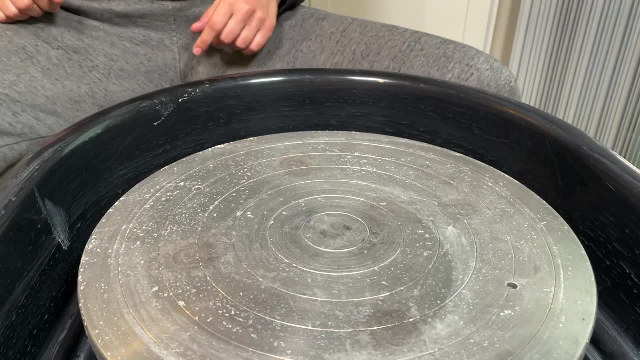 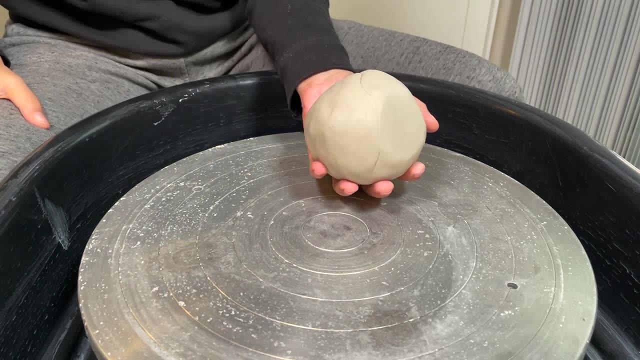 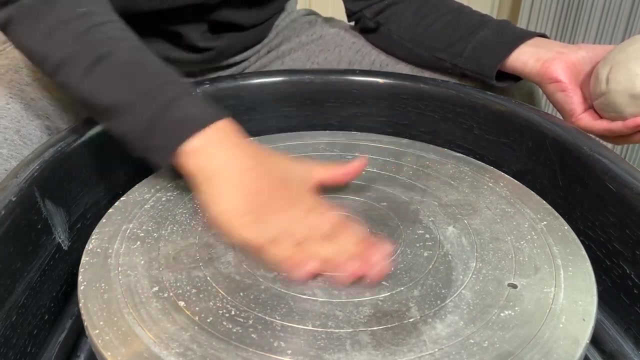 So the wheel should always be going into your palm. I have my piece of clay that I've already wedged. It's prepped and ready to go, And we want to first attach this to our wheel head. I'm going to use just the two drops of water We want to add just 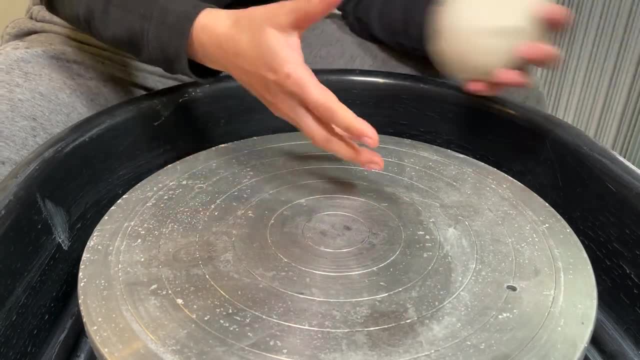 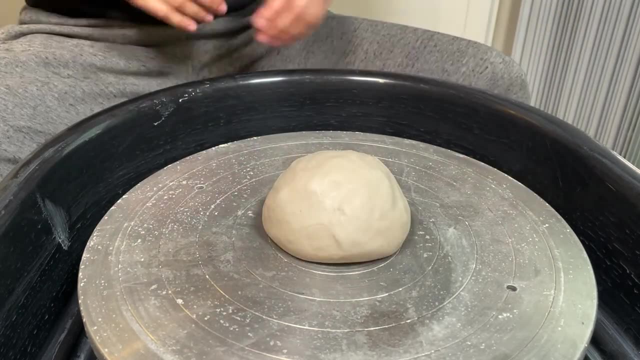 enough water to get this damp. We don't want so much water that our clay is sliding around. I'm going to go ahead and slam this down. I'm not setting it, I am slamming it down. You can see that we're a little off-center. No problem there. What I can do is rotate my wheel. 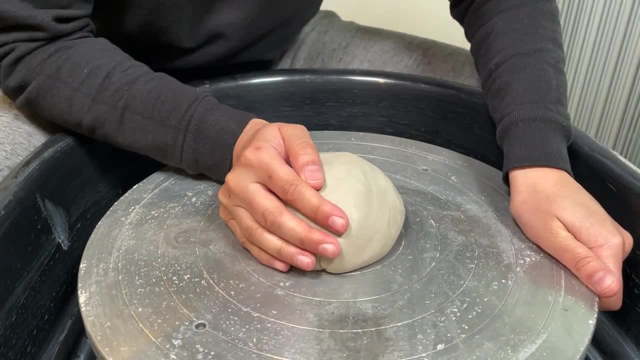 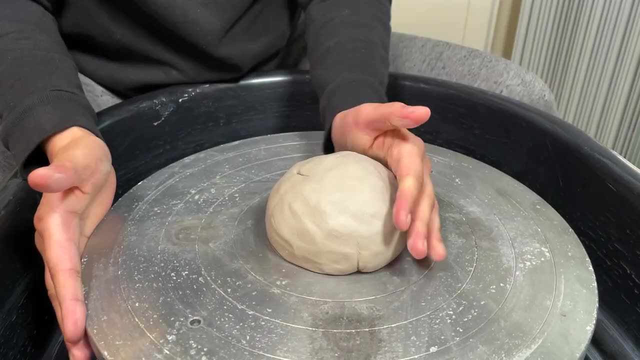 And I want to rotate it so that my adjustments are done by pushing the clay rather than pulling. I'm slowly rotating it. If I just try to push without any rotating motion, the clay might be harder to move. I'm eyeballing it. Once it looks like it's about center, I'll give it two pats on top. 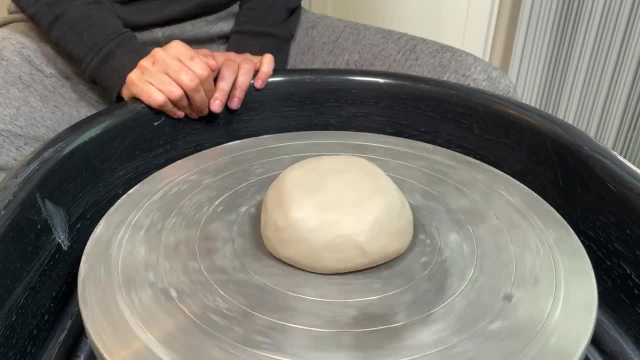 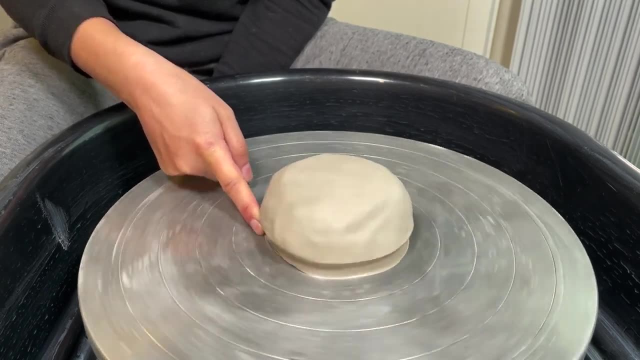 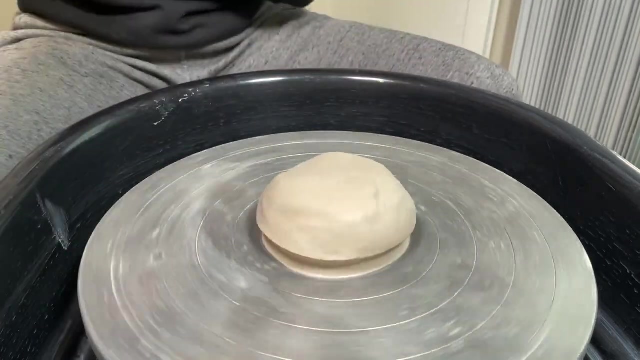 And I'll get my wheel just barely moving. I'm going to dip one finger in water And attach the clay all the way around, And what I'm looking for is to get rid of the seam. Once it's attached, I can go ahead and dip both hands in the water. 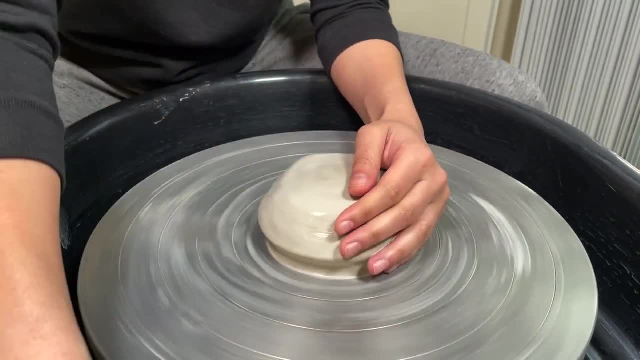 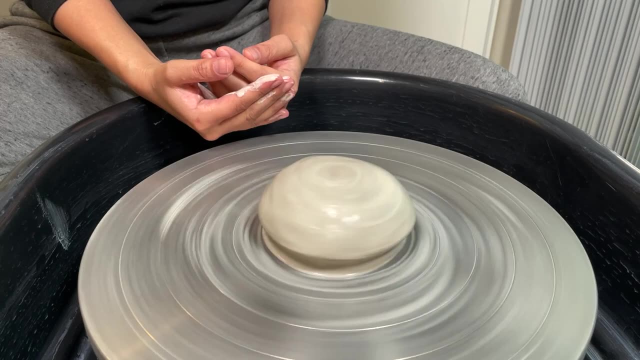 Get my clay nice and wet, as well as my wheel head, And then I can increase the speed. At this point, we've been at a low speed. We're going to go all the way, pedal to the metal. at this point, If we don't go at the fastest speed, it ends up being 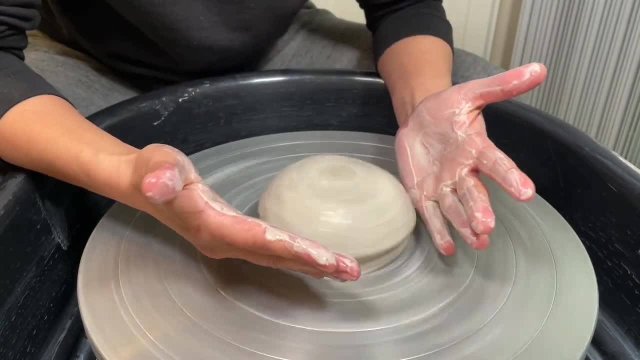 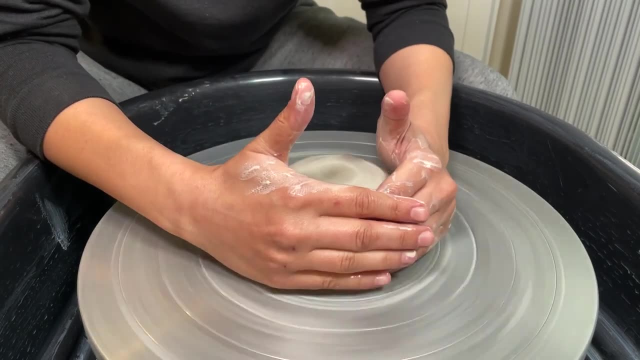 more work for us. That's a common mistake beginners make. You can think of it as you know. you have to hold the position longer, And so speed is your friend. The first thing we want to do is cone up How we begin to do that is by applying pressure on this. 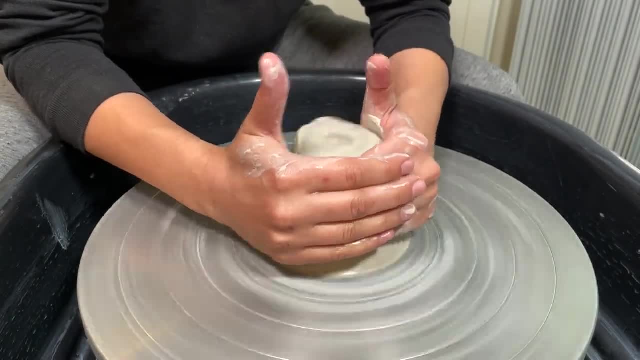 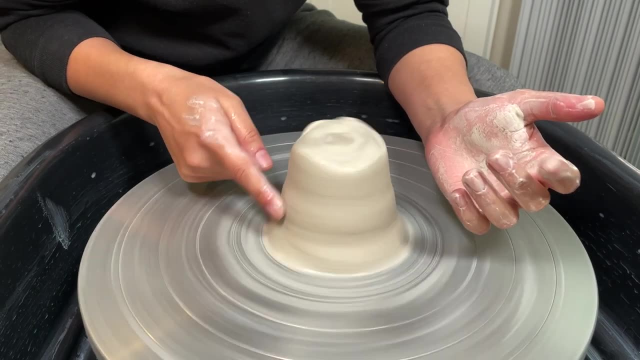 part of each hand, So it's our palm, and our fingers really aren't doing any of the work, They're just kind of around for the ride. You can see right away that the clay has gotten kind of sticky. so anytime it gets sticky or the wheel head gets hot, we're gonna get a little more water it. 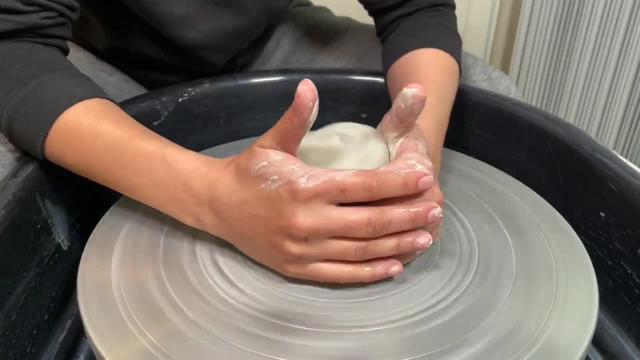 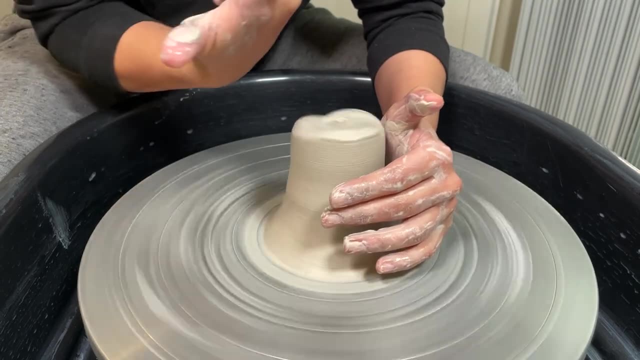 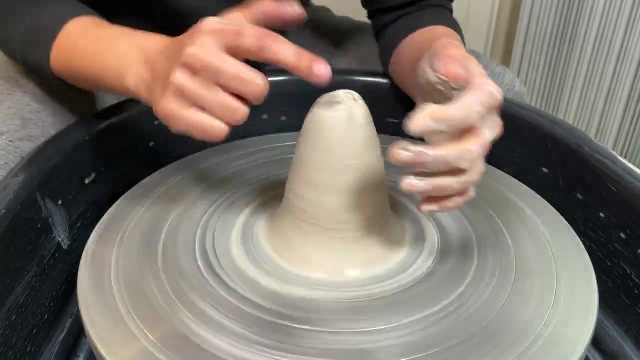 should always feel smooth and we shouldn't feel any heat. so again, coning up it's with the palms of our hand and pressure with both, you should see the clay go straight up between your hands. the common mistake beginners make at this point is by moving up the clay like this, and they end. 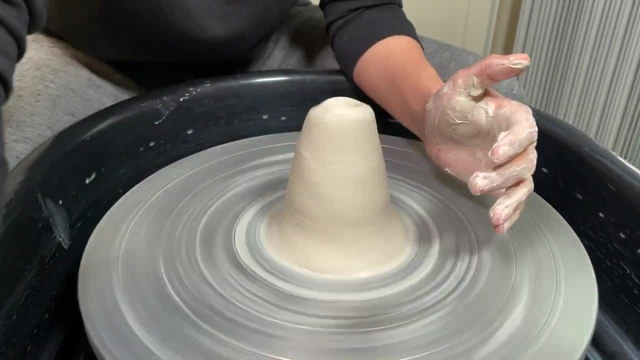 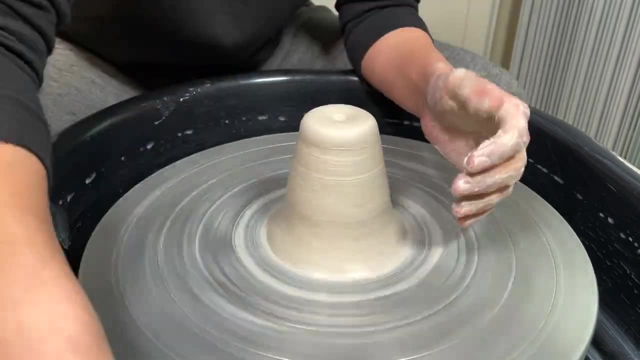 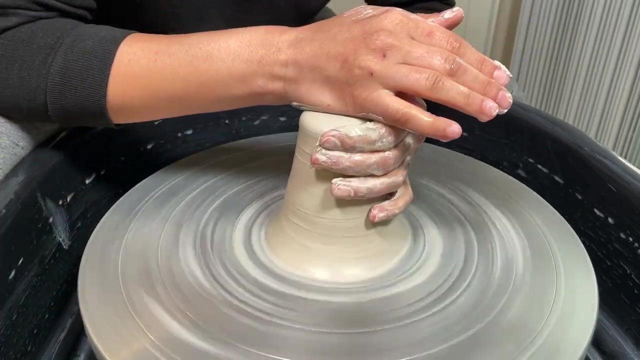 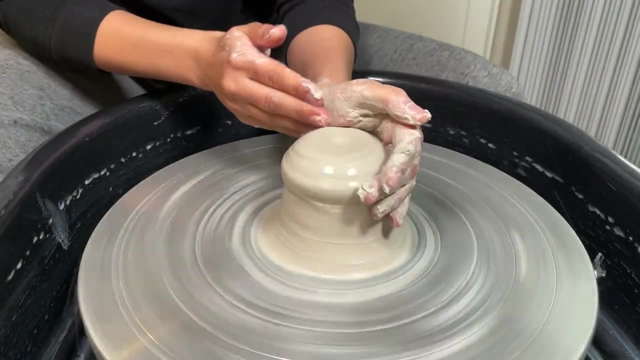 up creating a kind of a pocket like this to fix that. if that happens, you just want to start pressing it down without creating a pocket. but once we've combed up, we can go ahead and comb down. our dominant hand is on the top, slowly pushing down. the left hand is on the side, evening out. 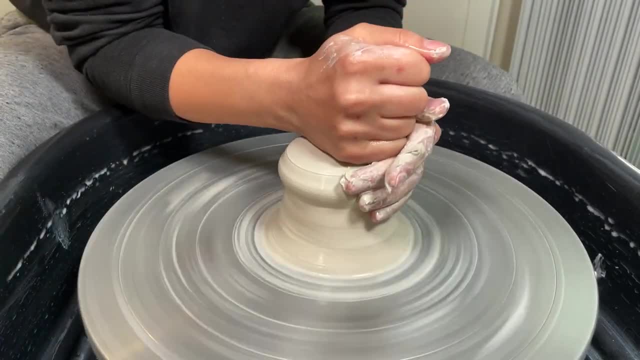 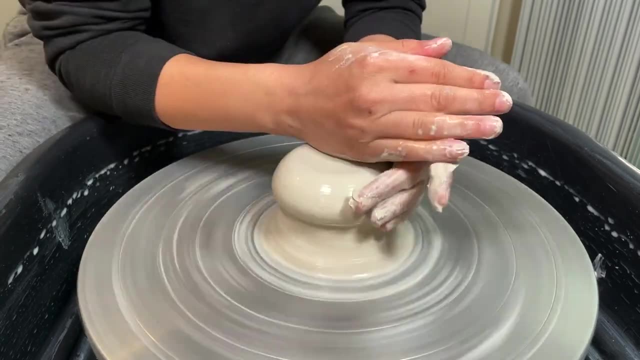 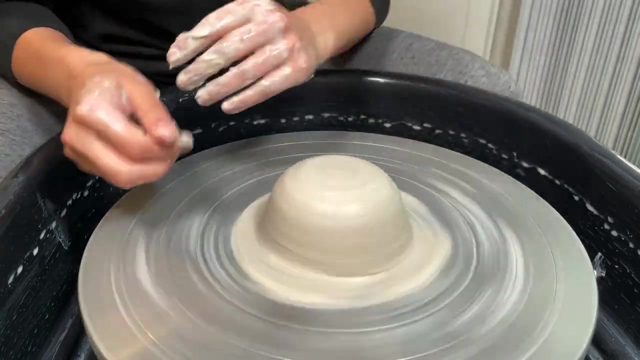 all the clay as it goes down and again, anytime it gets sticky, we'll grab a little more water. we're careful not to grab too much because the more water we add, the less time that we have to work with our clay. so we're going to continue to go down until everything fills in. this is a 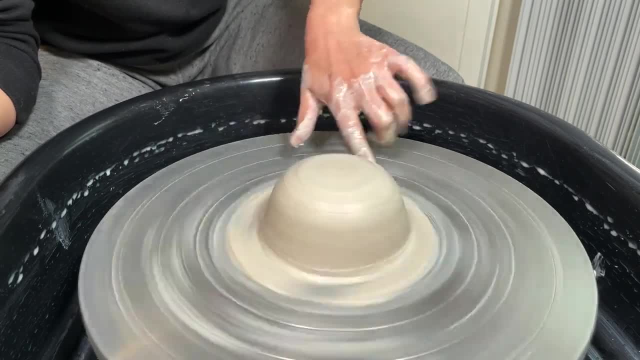 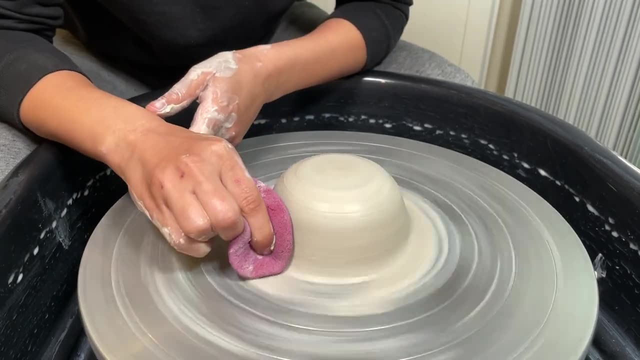 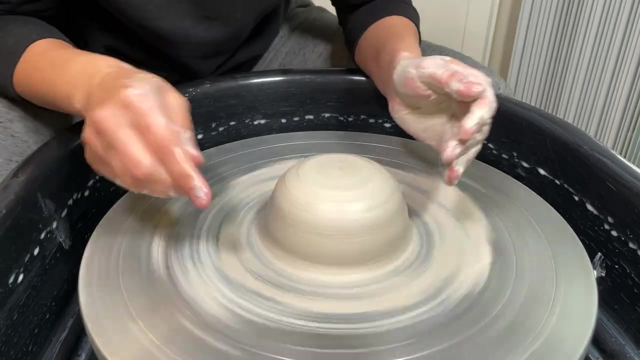 good opportunity to do a little sponge cleanup. this is super useful for beginners as well. you have your sponge taco in your dominant hand. elbows are on my legs for support. i'm going straight down right above the clay i want to get rid of, and now i can go ahead and get back to centering. so see, my clay could use a little at my wheelhead. 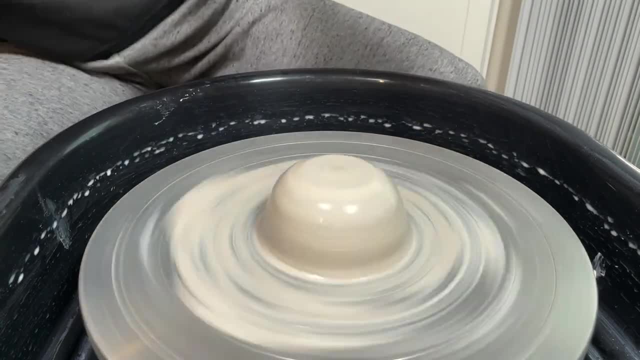 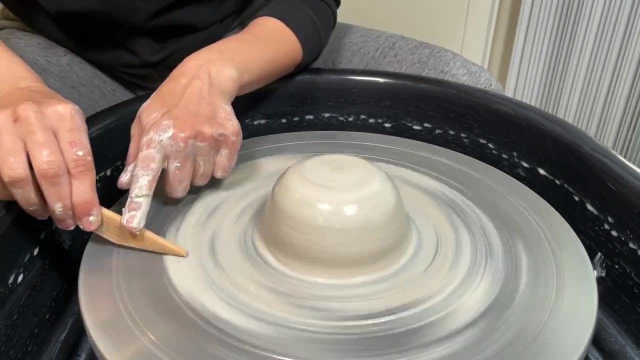 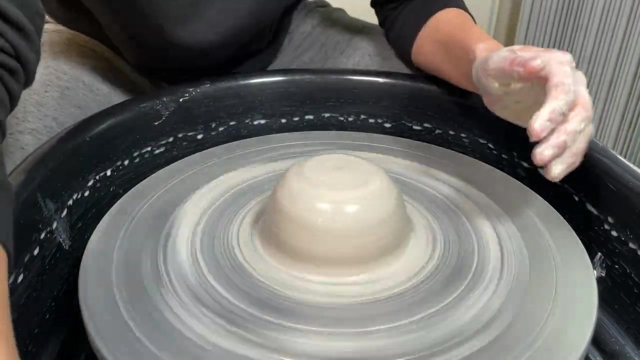 could use a little water. so anytime our wheel gets clay, we want to get that out of the way. using the blade side of our wooden tool, i'm pressing down with my left hand. my dominant hand is holding the tool and now we're ready to finish centering. so from here, anything on. 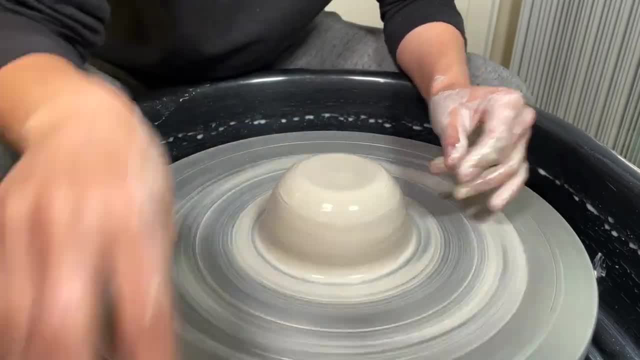 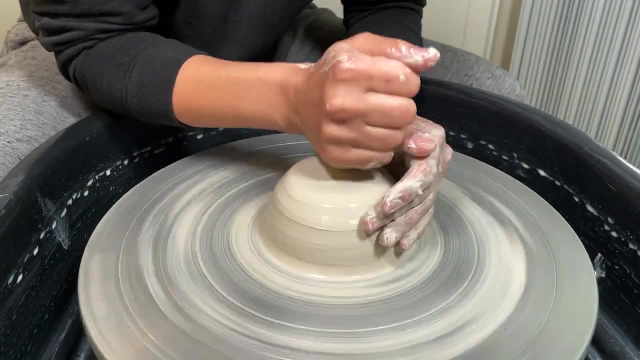 the top will be taken care of with my right hand, because i'm right-handed, and anything on the side will be taken care of with this part of my palm, because we're going to be throwing a bowl. we're gonna. we're pretty close to where we want to be. we're just going to even it out. a common mistake. 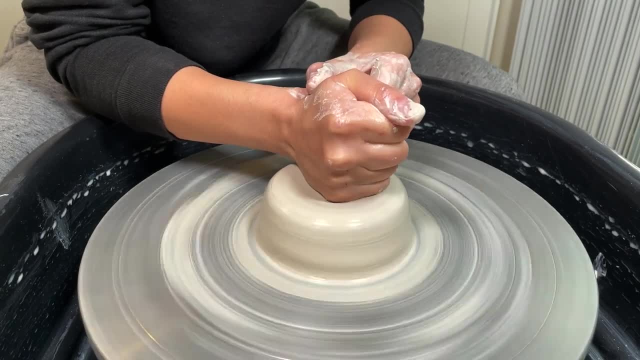 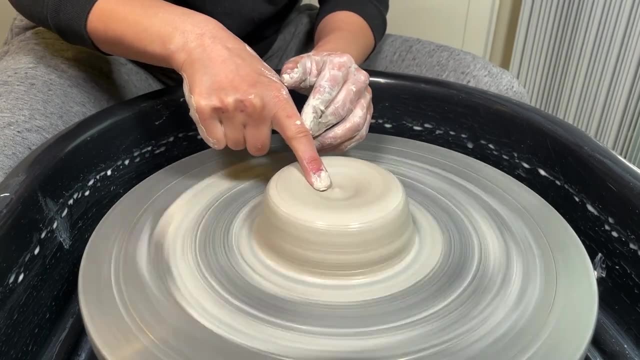 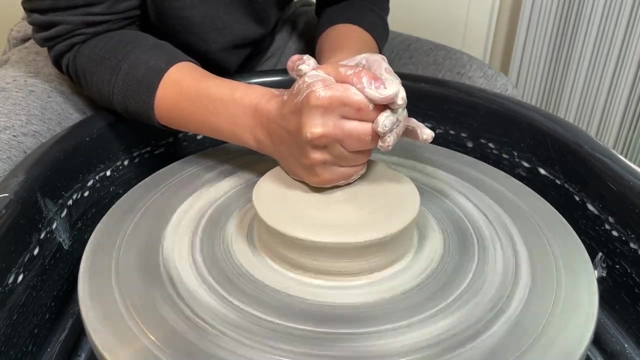 here. that beginners make is they'll apply pressure to the center rather than right here in front of your belly. uh, what that ends up doing is creates this little. it creates this little pocket that we don't want. we want it to be level. so if that happens, shift your hand a little lower, so it's. 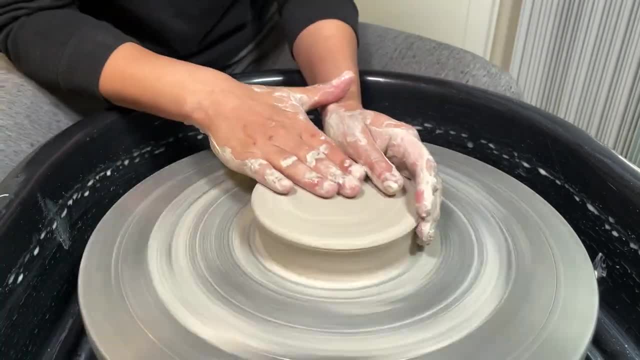 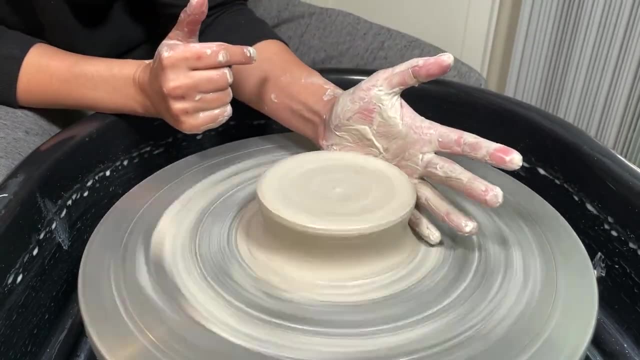 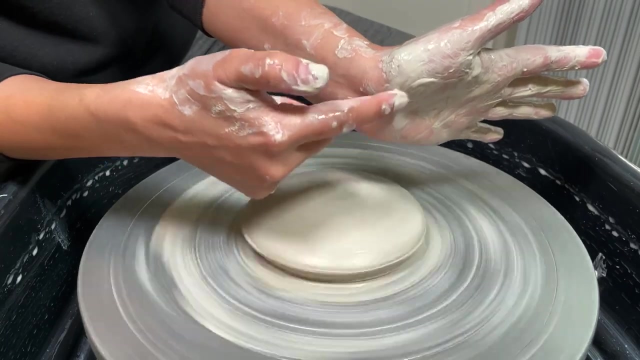 about right here. that's how you'll get a nice flat top and a common mistakes. with this left hand we'll see we'll kind of adjust their hand too far this way, so you'll get a little mushroom top. sometimes the hand can be far too far in, so we'll get a little flapping. what we want to do is be. we want to be. 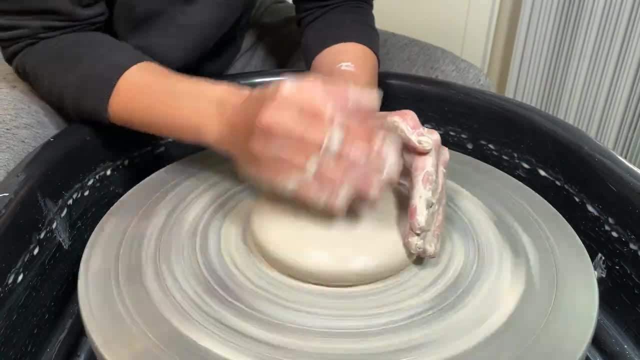 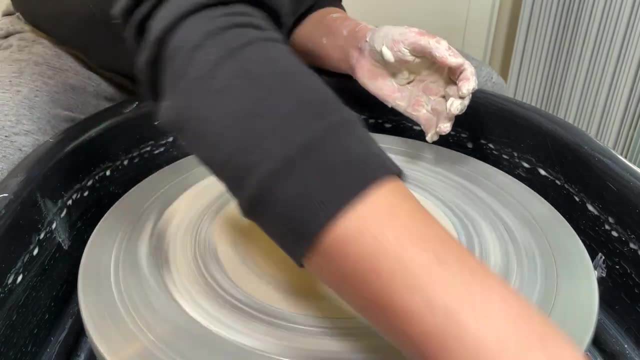 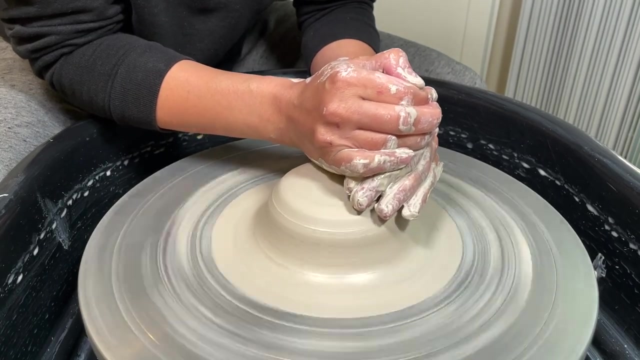 right about here. so what that looks like is when we do everything together, we're going to get our clay nice and even, and how we can tell that we're all done. centering is if we rest one finger against the side and it doesn't bounce, we're good to go anytime we're letting. 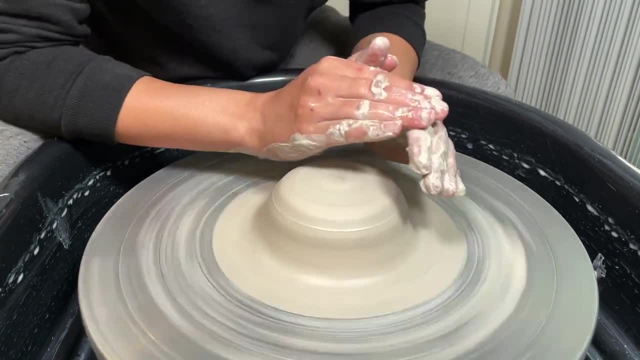 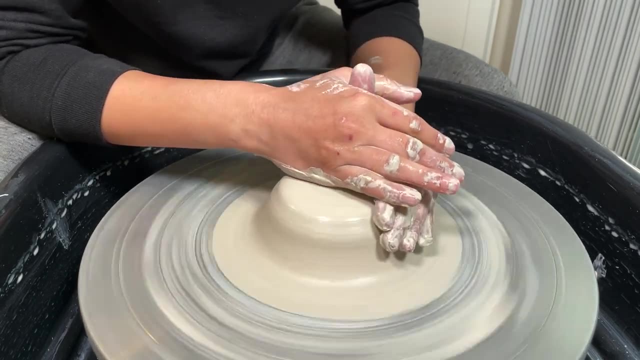 go of the clay. it's a gentle release. if you're wondering what happened when your clay felt centered and all of a sudden it got knocked off centered, that could. that was likely. what happened was just that you let go a little too quick. um, you want to think of each cycle? 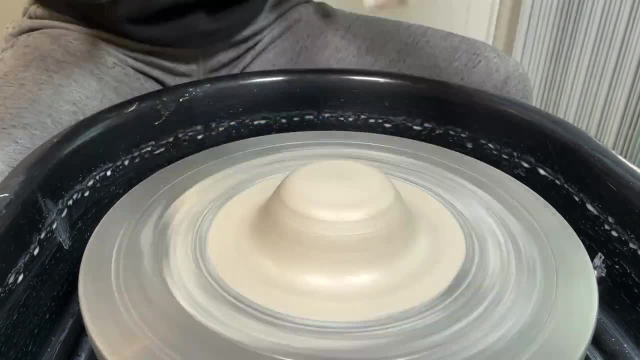 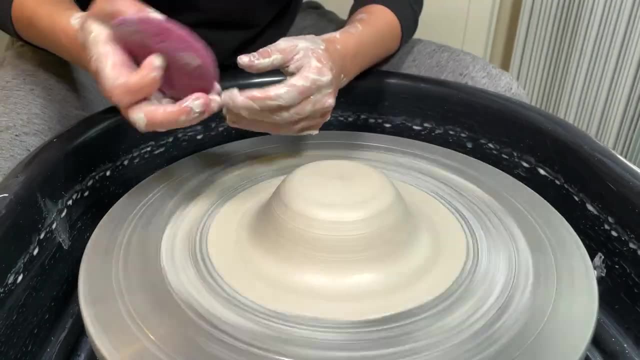 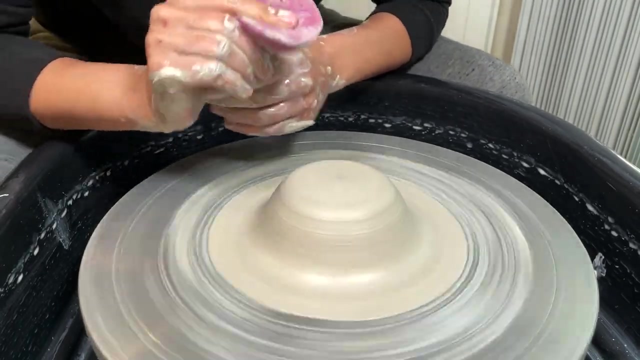 and make sure you release accordingly. so that's why, again, the speed is on your side. from here, we know we're all good to go, so we can go ahead and get our sponge taco In my dominant hand. I'm supporting my right hand with my left, elbows are on my leg and 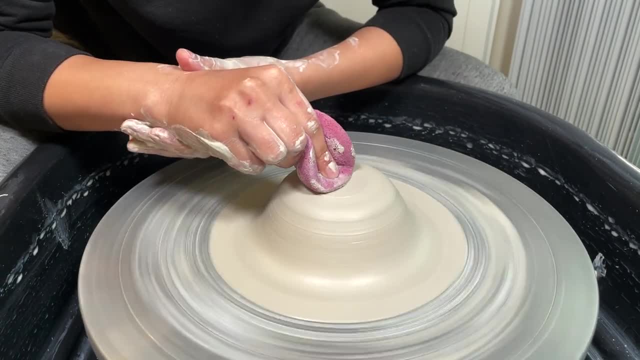 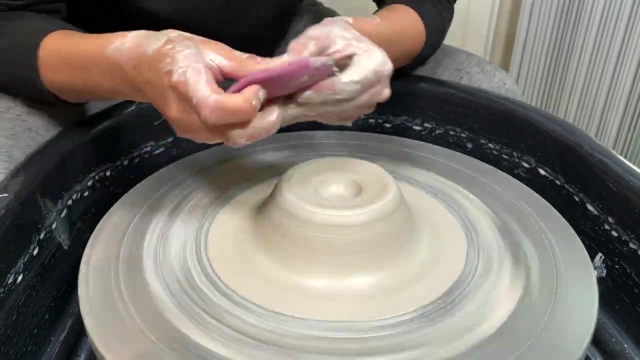 my nose is right over the center. I'm going to start by pushing down. And a common mistake here: beginners might go a little off center. what you can do is kind of get to a clean side of your sponge and start again and keep going down. 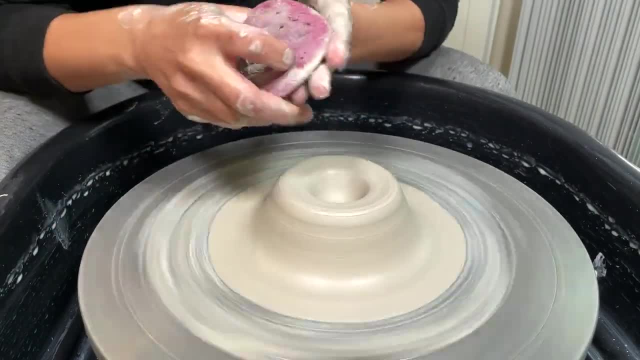 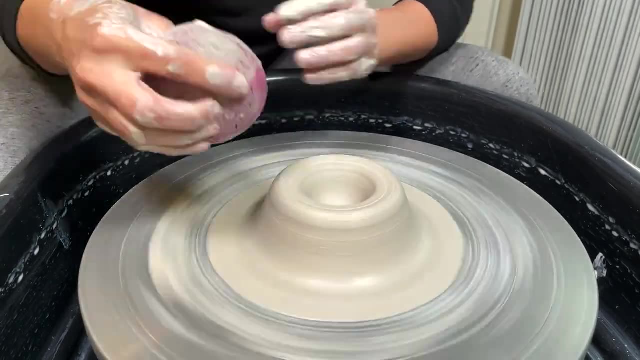 You want to remove your sponge and see how far down you've gone. We're aiming for about half an inch at this point. You want to be careful not to go all the way through, because what we're doing at this point is creating the base of our bowl. 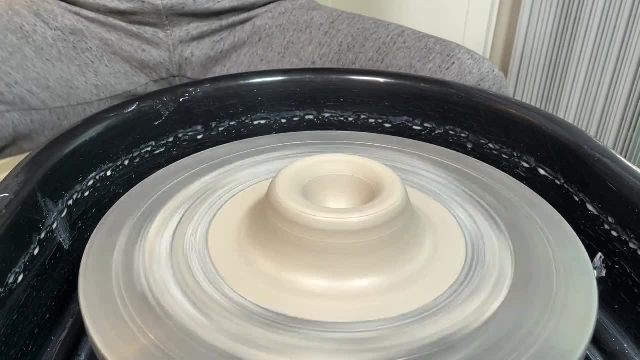 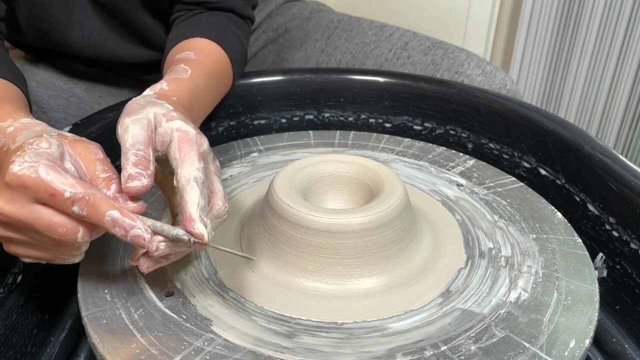 When we think we're about there, we can go ahead and get our wheel off by pushing down on my foot pedal. I'm going to go ahead and grab my needle tool to see exactly how much clay we have on the bottom. I'm going to make sure my wheel is off so I don't accidentally cut a hole through the. 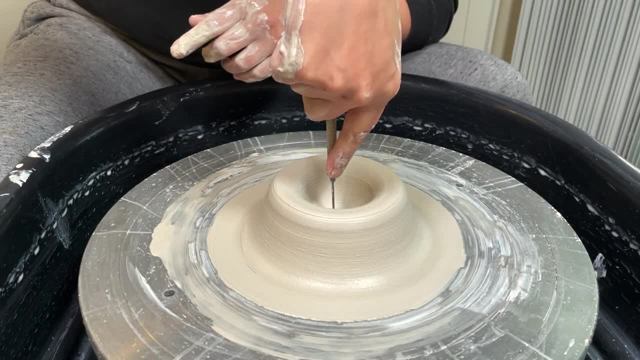 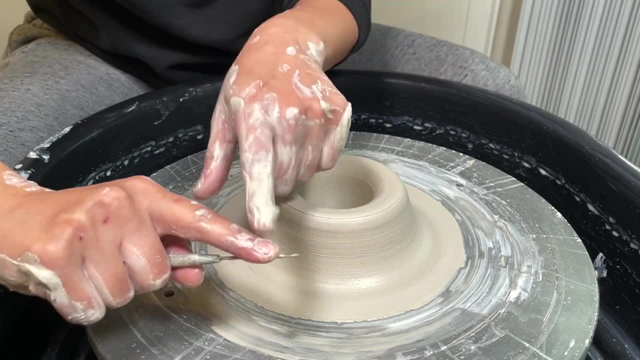 base. Put my thing, my needle tool, through, slide my finger down until I hit the clay And lift up and I can see that we're where we want to be. if we're not going to be trimming our foot yet- which is what some you know- that's not a bad idea for your first bowl. 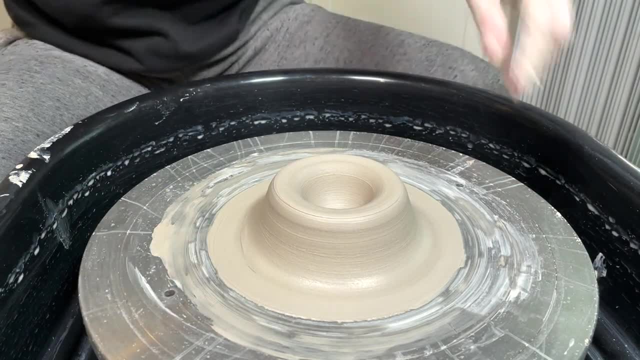 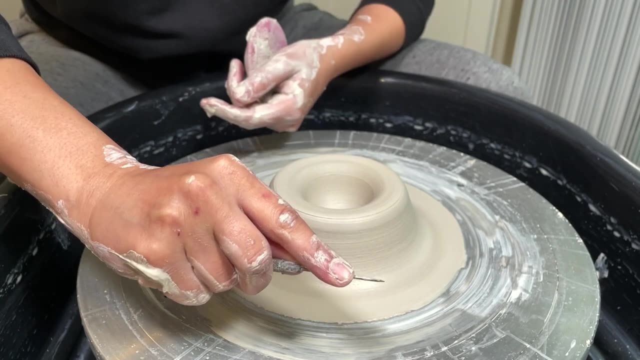 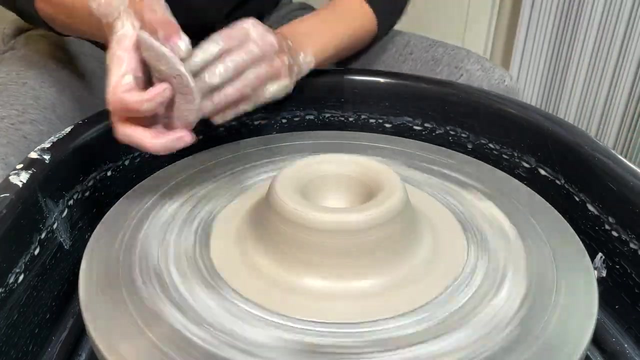 We'll save trimming maybe for the next one, And so if we were trimming somewhere, about three quarters of an inch is where we would want to be right now We're closer to half an inch, So we're going back to full speed. I'm going to press down. 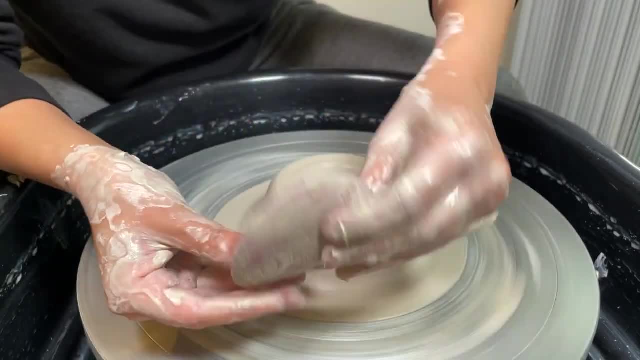 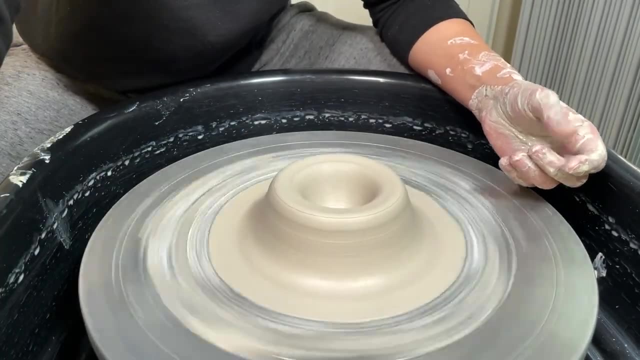 To get rid of that needle mark. Whenever my sponge gets like this, I'm losing control. it's sticky, So we want to go ahead and make sure to clean that out fully. It'll help my grip and I can get more control. 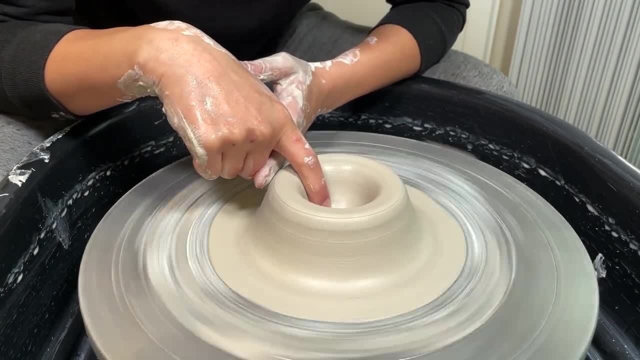 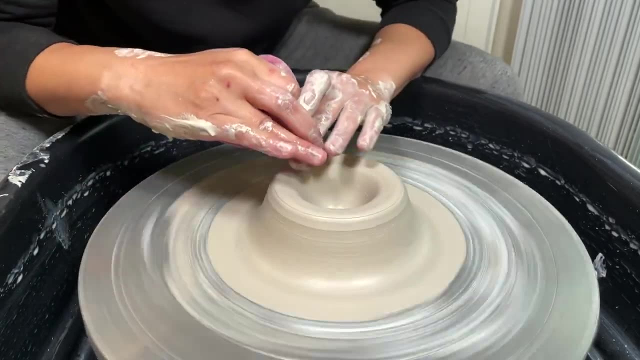 Another common mistake beginners make is- well, we all make- is, you know, going down a little too far can happen. This is the step where we can fix it. Once we've stretched out, our floor is going to be our floor, So we're going to go ahead and get rid of that needle mark. 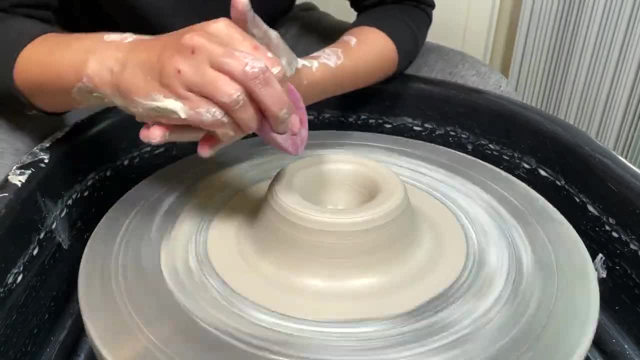 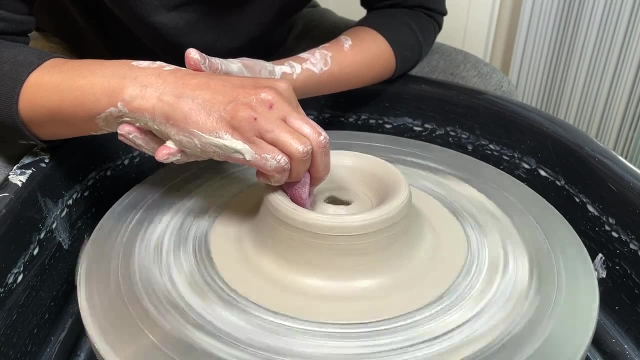 If you want to do anything, it would be an additive. you know, with flipping and scoring. So here you can actually create a ridge and start pushing that down. But you want to be careful not to create a giant air pocket, because air pockets will. 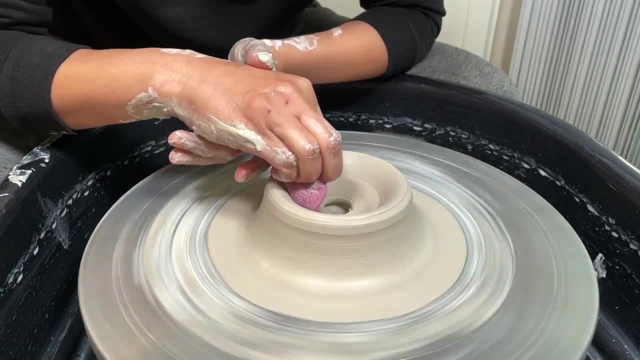 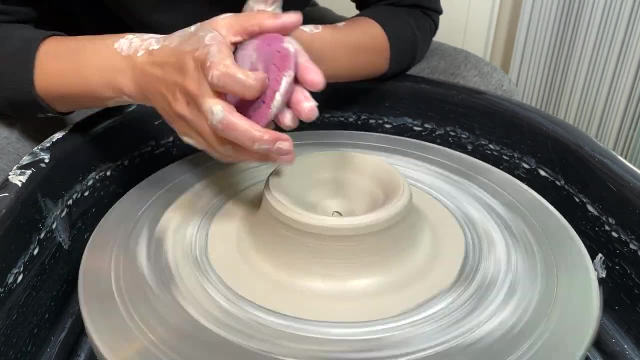 explode in the kiln. So what we're going to do is go back and forth between this ridge and pulling that out, And that's how we can. if we for any reason end up going a little too thin and we need to fix that, we can mend it like so. 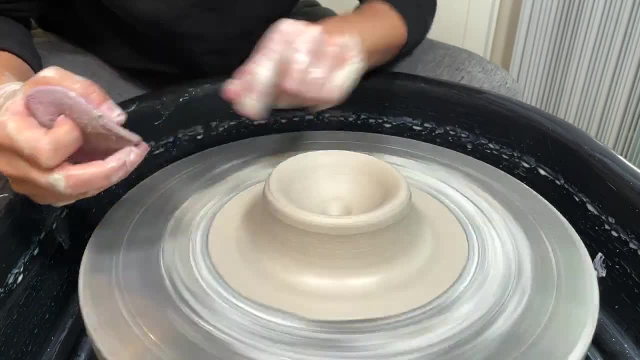 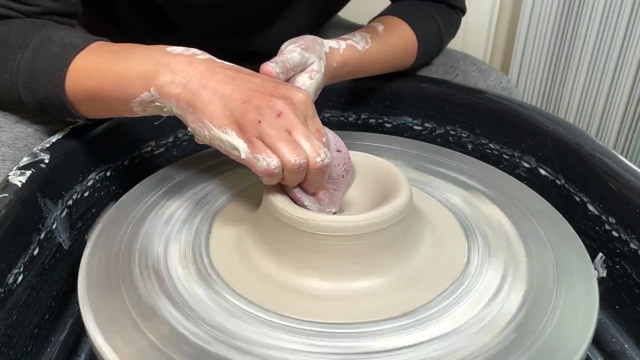 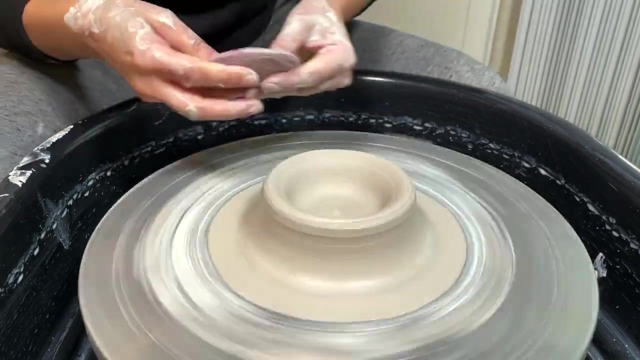 And that's it. And so you can see that there's no possibility that we created an air pocket, because we kept it clear all the way down. Now we can compress and blend in, And that's a quick way to save your bowl. Now that we've measured it, we can go ahead and compress. 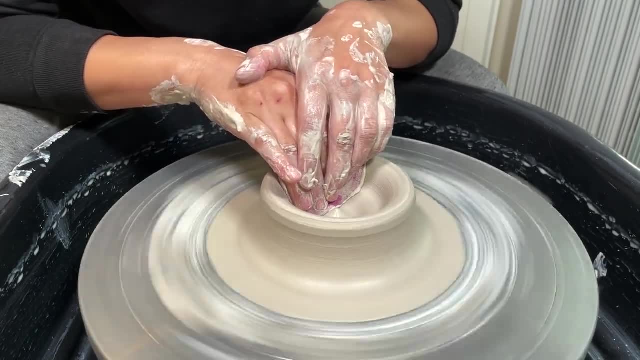 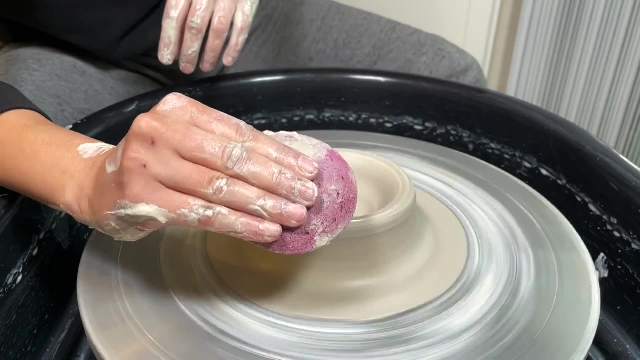 And we're ready to start pulling out our piece. So what we want to do is use the fingers to pull and how our sponge is set up. So we're going to go ahead and do that With our dominant hand. we have our fingertips over and then our other one goes over as well. 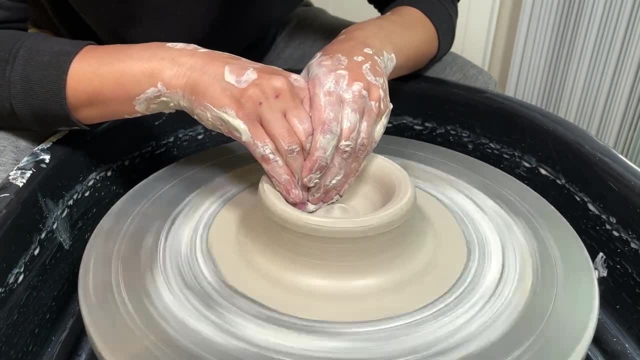 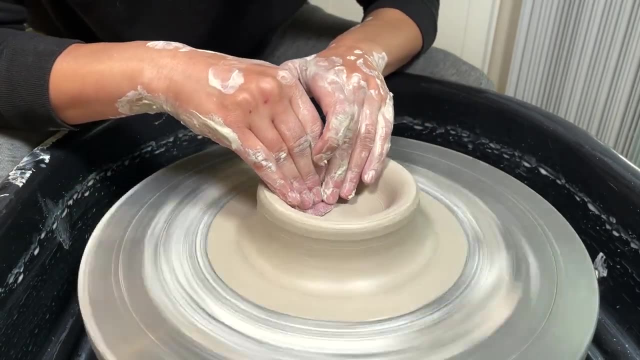 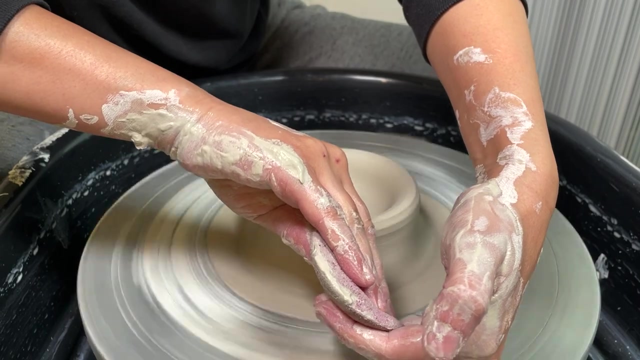 And we get our sponge into our piece and pull towards our belly button. Common mistakes: at this point we often see. you know, we don't want to pull out too far, but the angle of our fingertips will make a difference. So if we angle it this way, we end up with the slope. 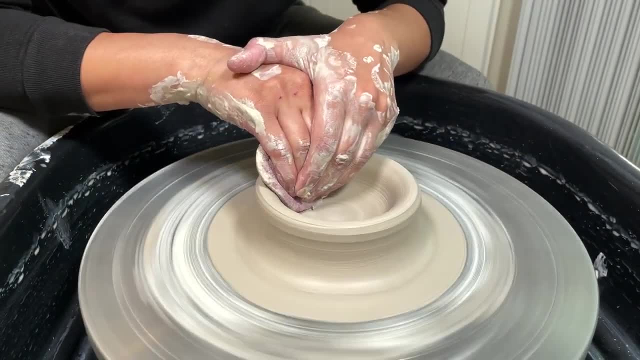 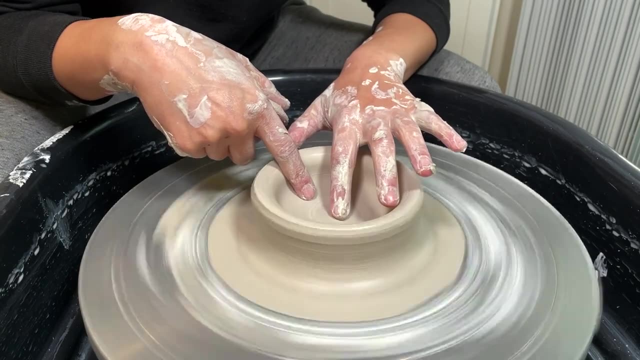 If we tuck our finger in, we really get a nice wall to work with for our next step. So that's pretty much it. We're kind of closer to what we're going for At this point. we've pulled so much clay we're very likely to get an S-crack. 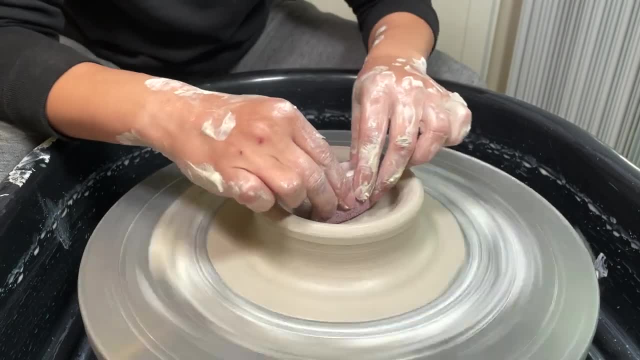 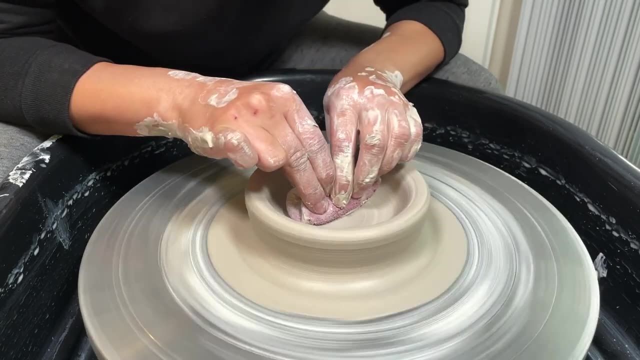 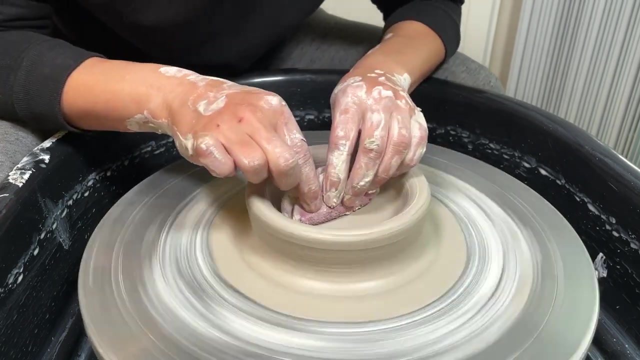 So to prevent that from happening, we're going to fold our sponge in half, compress against the base and slide over to the right until we've hit everything. It never hurts to go over twice. The last thing I'd want is for you to have a crack after you've gone through all the steps of getting your beautiful piece. 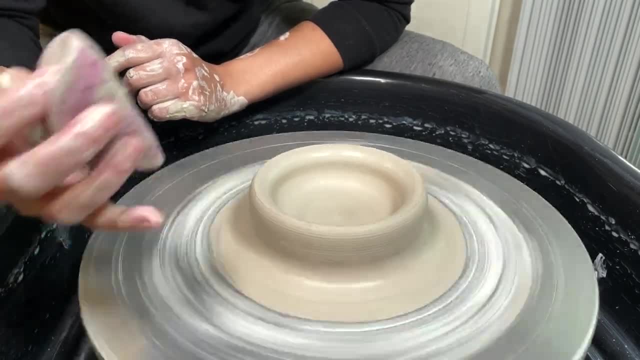 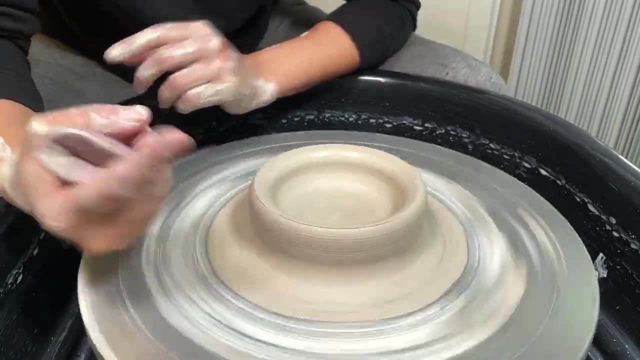 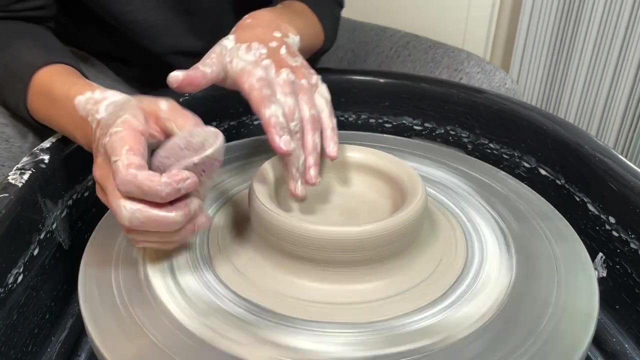 on to the next step. i always recommend this housekeeping step. we are going to be pulling a cylinder next, um, with any, any shape you make on the wheel. the foundational steps are centering, opening it up, compressing the base, pulling the walls and then shaping, trimming the lip trimming. 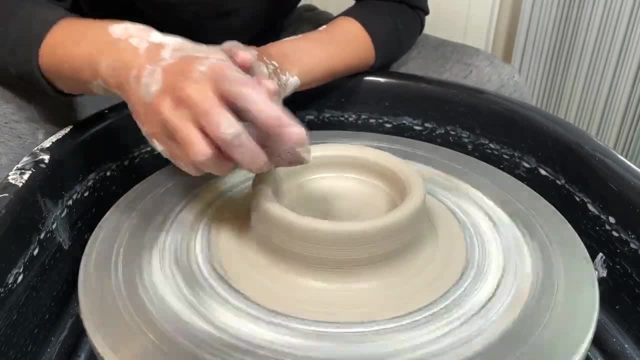 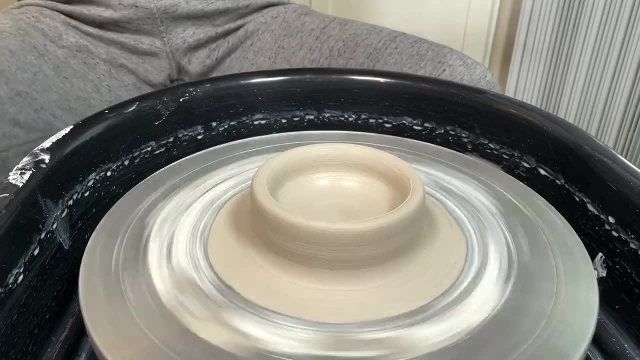 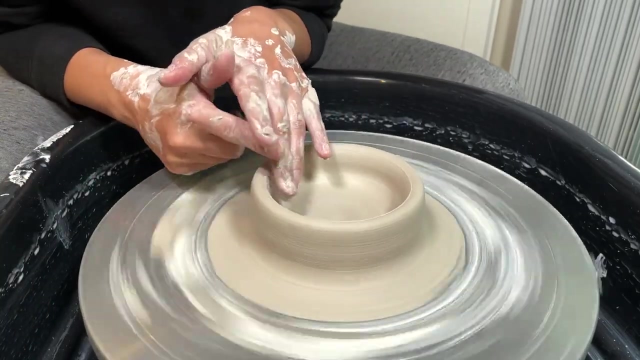 our foot, but what we want to do is do our little folded sponge housekeeping. that's going to set us up, and this is when we're going to get down to medium speed and we're going to make sure our sponge is as clean as possible because, uh, i would say, along with centering, pulling our walls can be. 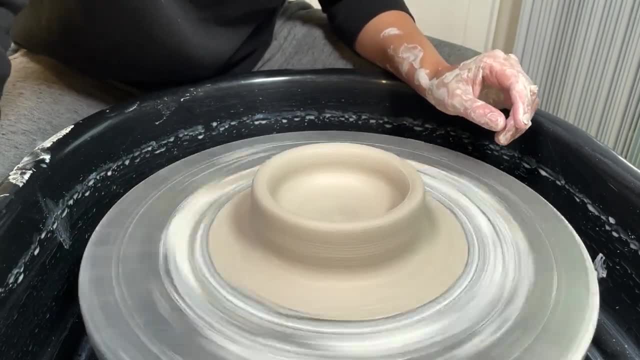 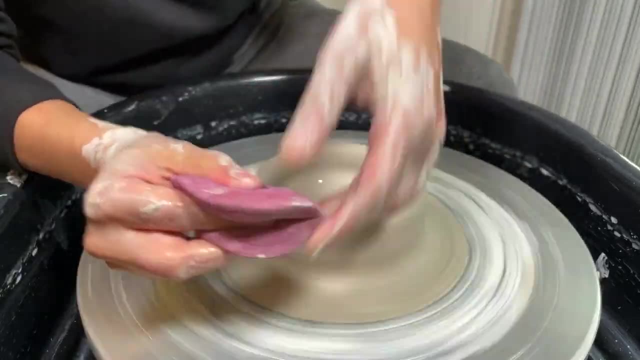 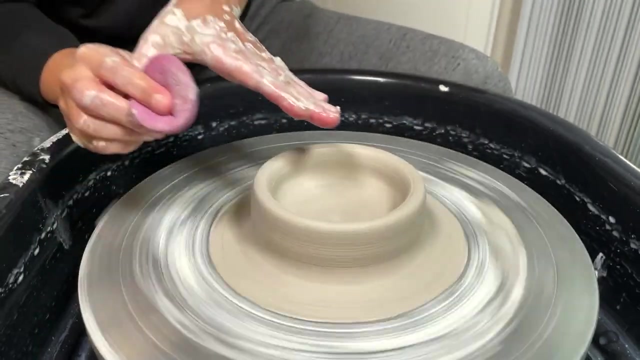 one of the trickier steps when we're just starting out. so with our nice and clean sponge, we will get our sponge taco. i'm going to go ahead and wet my fingertips in my left hand and string my left thumb through. my sponge is on the outside and my fingertips are on the inside. my elbow is on my leg for support. 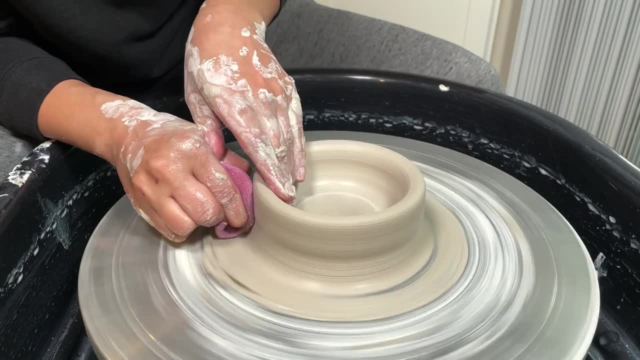 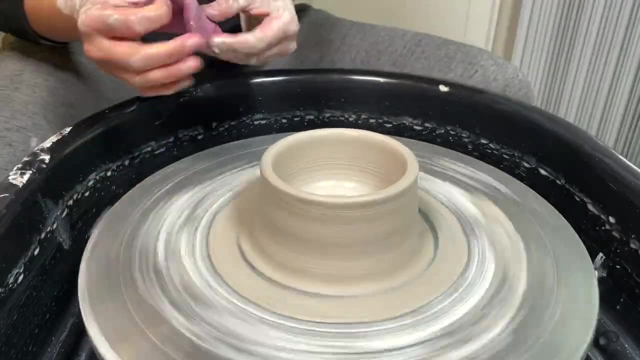 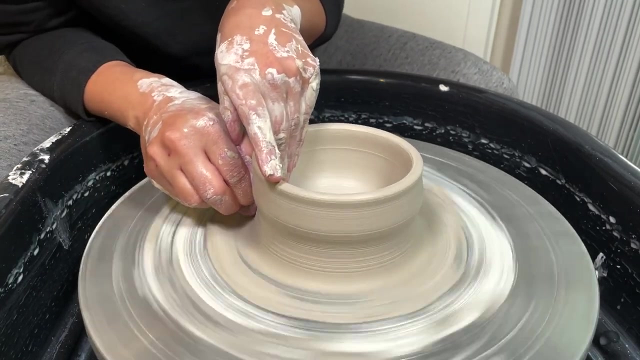 and i'm compressing against the base and then pulling up slowly, and this is when we're paying attention to the thickness of our walls and the foot. this is the time where we can get that the way we would like, so sometimes the clay can kind of feel. 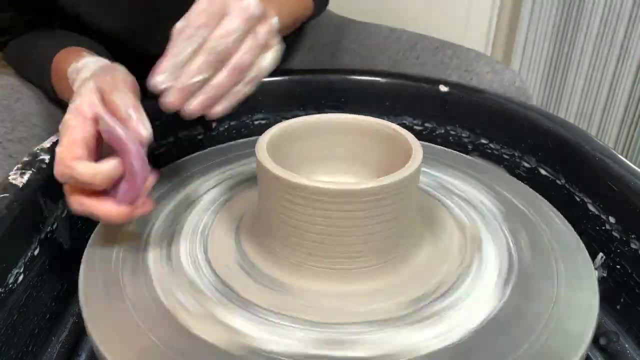 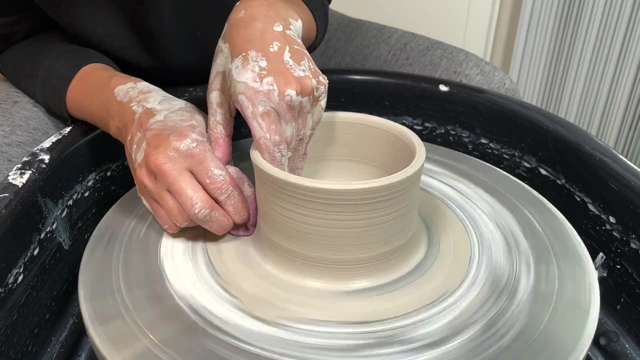 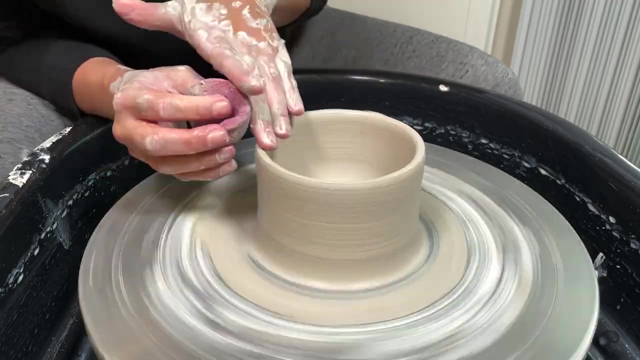 stuck towards the foot. the way we can correct that is by spending a little longer on the base and waiting till i build that ridge and then taking that up to the side, and that's how we can prevent having kind of a thicker base and, uh, you know, a thinner rim. we want it even throughout the 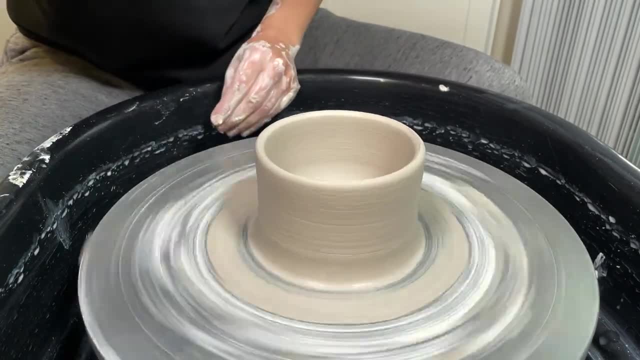 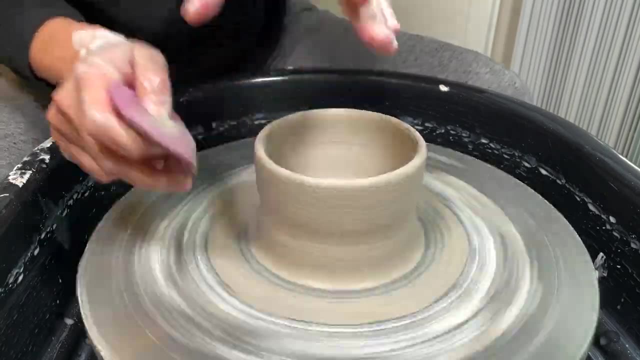 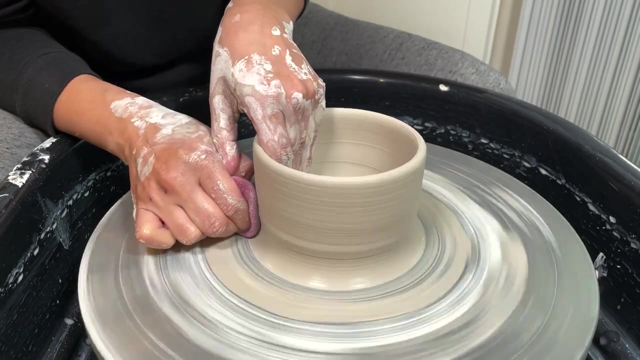 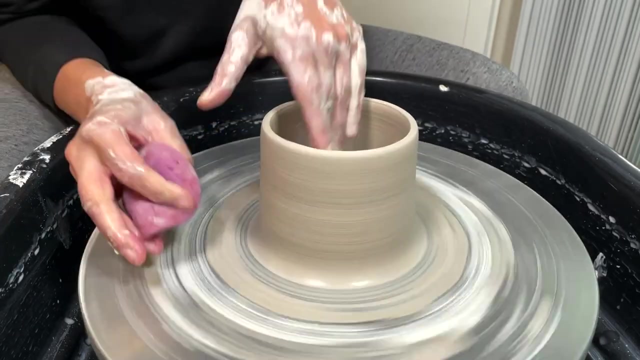 whole piece. so i think i'll give this one more pull. i am again cleaning my sponge because i don't want to risk it catching up. off this piece is the fingers on the inside sponge, on the outside i'm compressing and slowly pulling up. we're not worried about our lip getting wonky. that can um happen when we are evening out our walls. 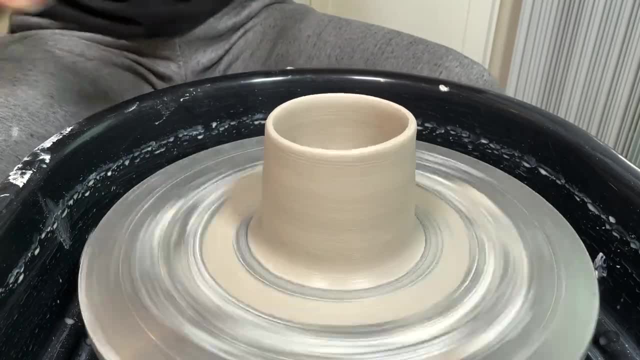 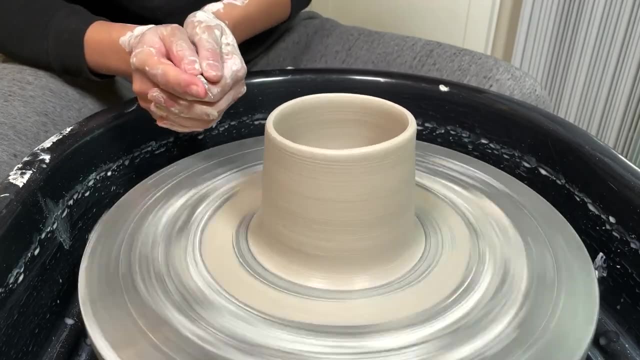 especially when we first start throwing. but we can come in with our needle tool and trim that right up. there are a few ways to trim. one is you can hold it if you're confident, your walls are nice, and even this is a great way to go. you can hold your needle tool with both. 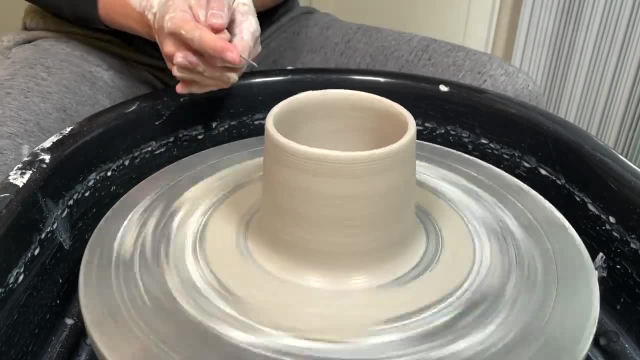 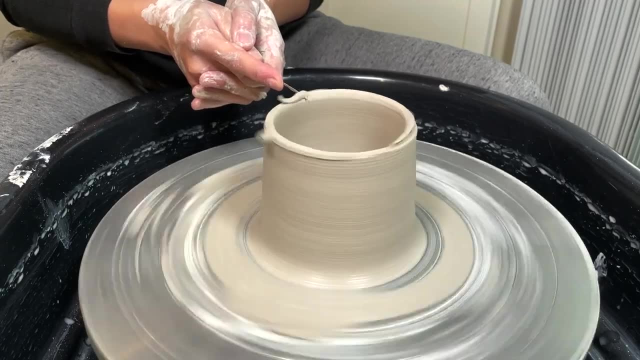 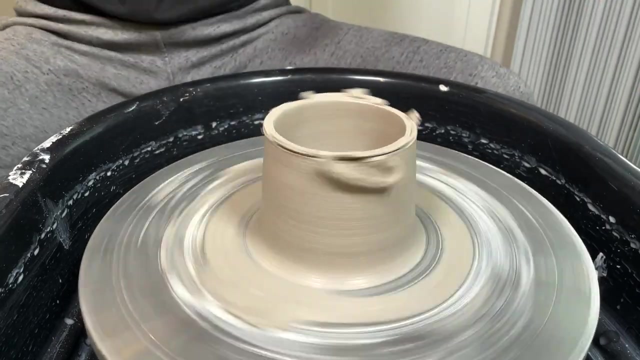 your hands, your elbows are nice and tight against your side so you have more control. you don't want your needle tool wiggling. it needs to be nice and tight. you're going to start from the side, go through and then lift up and if it gets stuck like that, which can? 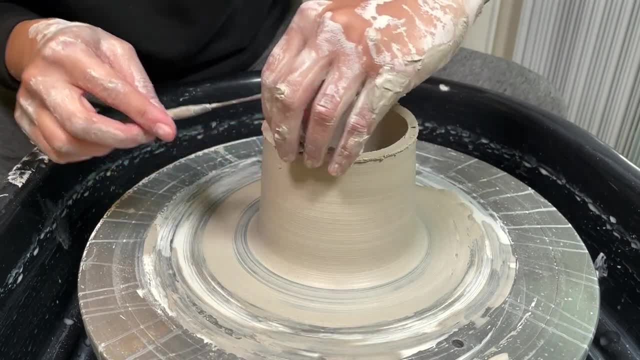 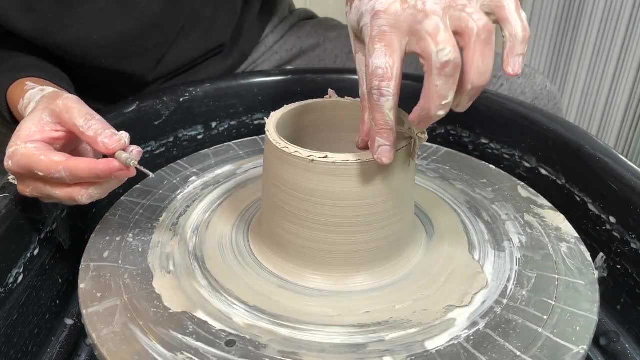 often happen when you first start. you want to get this off and all these chunky pieces you can pull. you don't want to go in with your fingertips because they'll push it in more. so this is a good example. i'll grab it from the top and pull that right off. 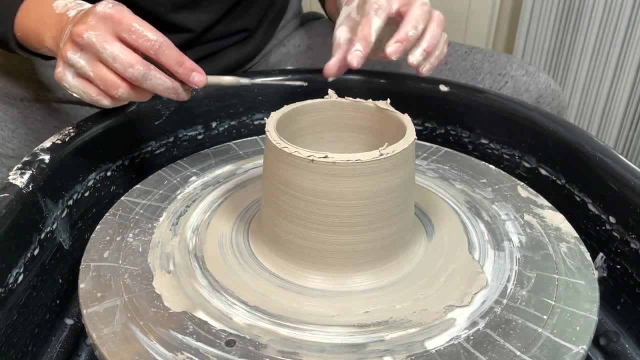 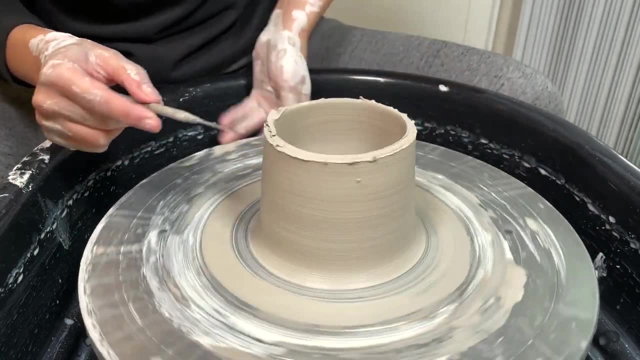 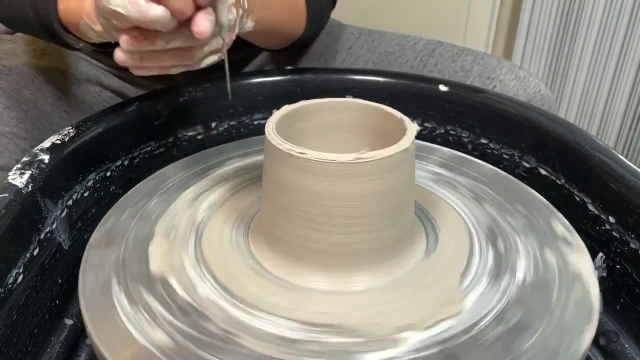 and any of these pieces will want to get rid of something like that. i can blend out. this is something i want to get off. so you can see, i use my needle tool. i don't use my fingertips um stuff like this. i might just go in with my needle tool. 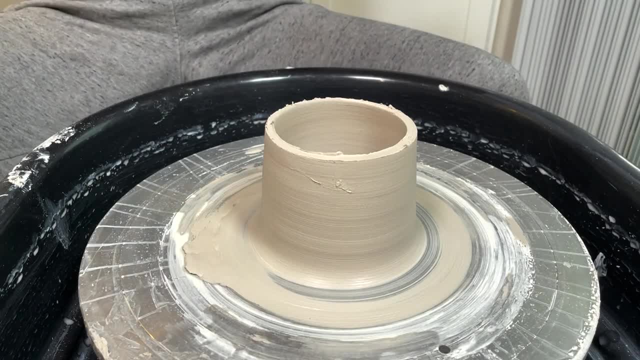 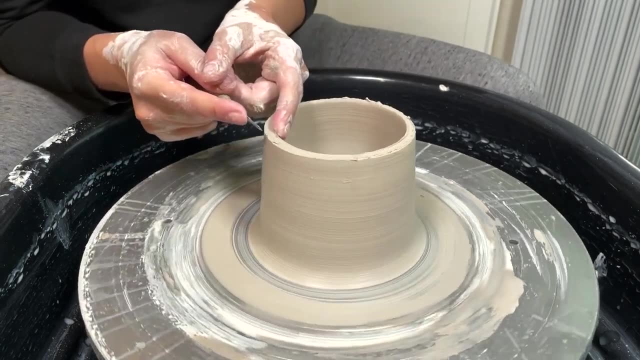 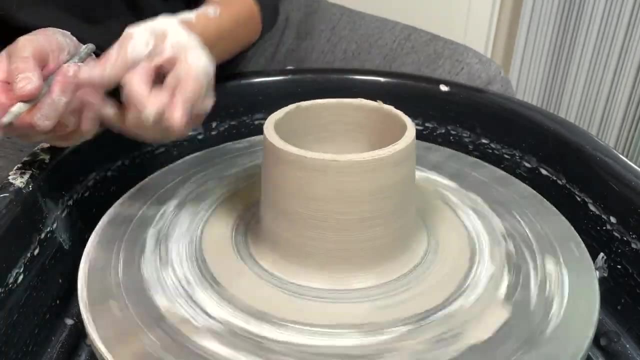 just to make it a little quick cleanup. and so the other way i recommend trimming is, if you this one, uh, you're not comfortable with, or you feel like your walls are a little thin and you need a little support, go back to medium speed. and how you can trim that way is with one finger that's wet. 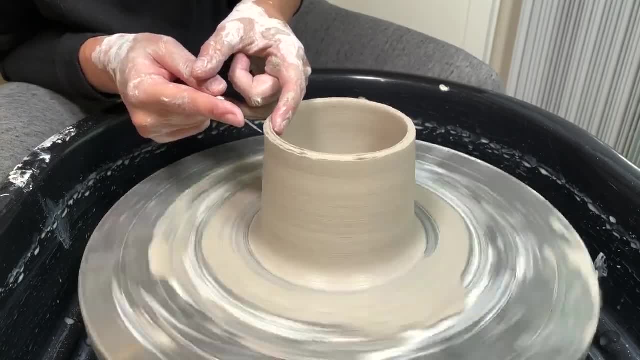 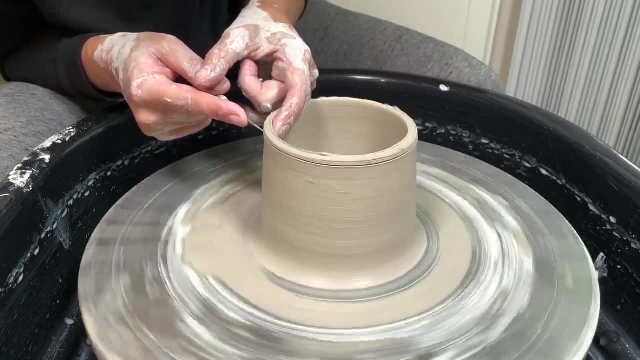 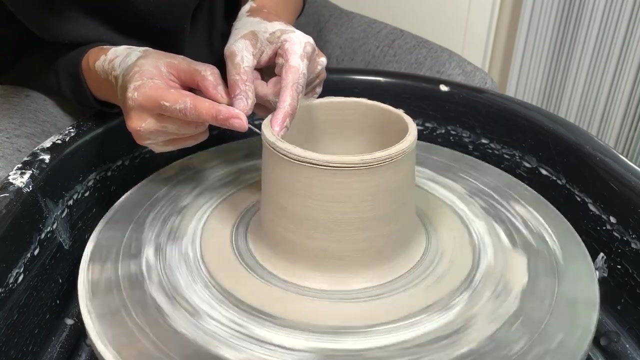 so it can glide along the inside and then our needle tool will slowly go through. um, beginners will often feel the needle tool kind of. you know we lose control. a good way to prevent that is by first sketching our line in and then going through. so hold it there and then go all the way through. 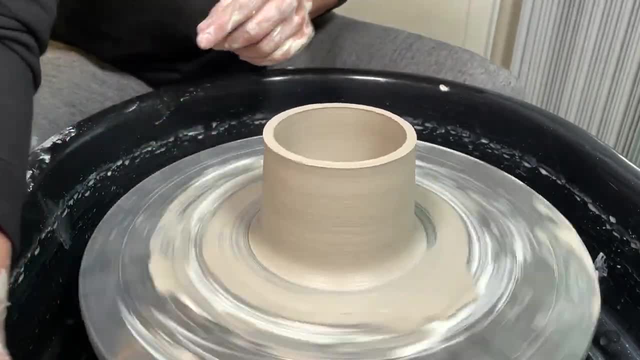 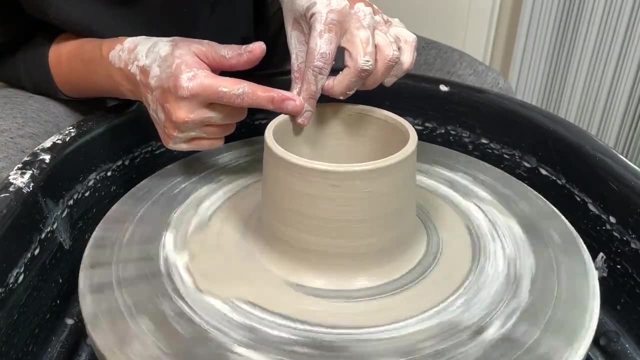 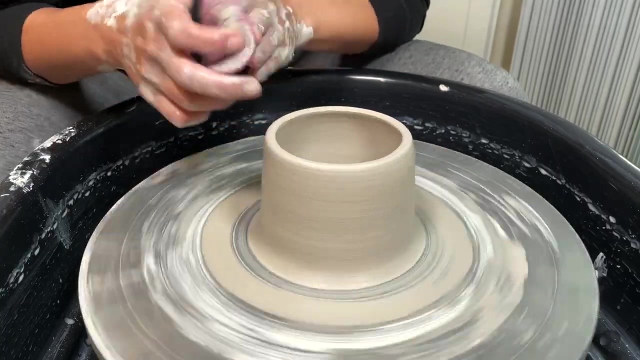 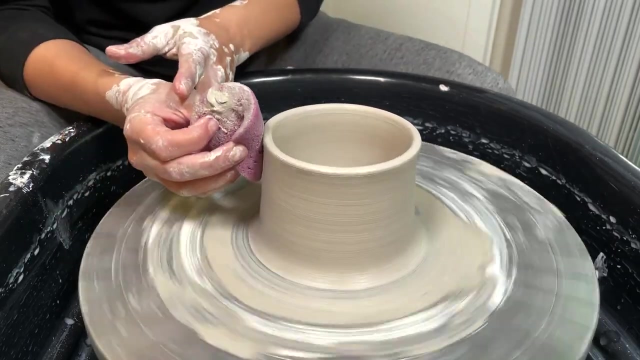 and then lift up and to clean this up and round out our lip, we can wet these two fingers on our left hand and then our right one is on top, or you can go in with your sponge, and now we're ready to start shaping our bowl with this one. you'll want to grab your wooden rib tool. 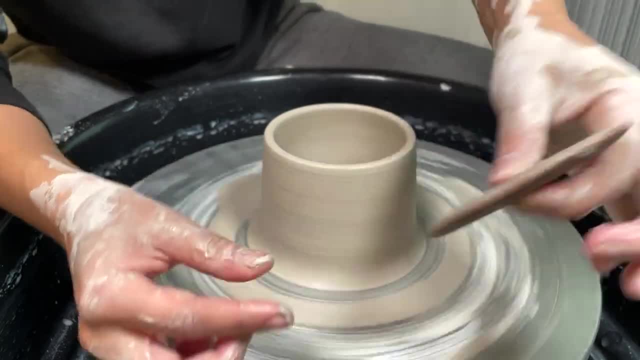 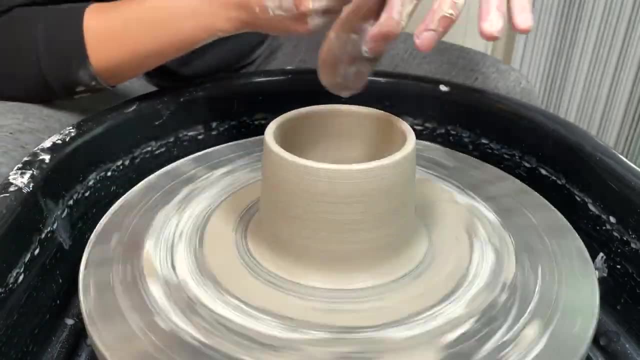 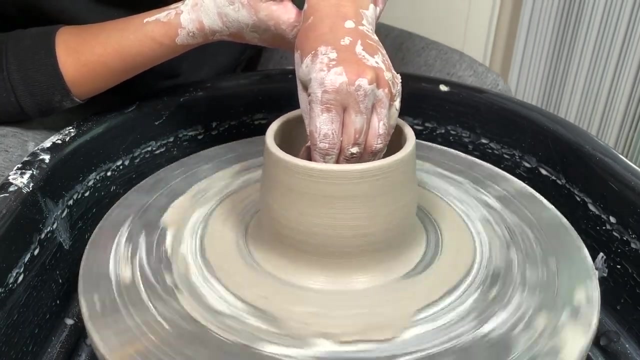 with the circular, thicker side facing the base, and this will be held in your left hand. we can go ahead and dip our tool so it slides up the side and our left hand is supported by our right elbows on my leg and i'm going to apply pressure to the wall, starting from the base and slowly making my way up. 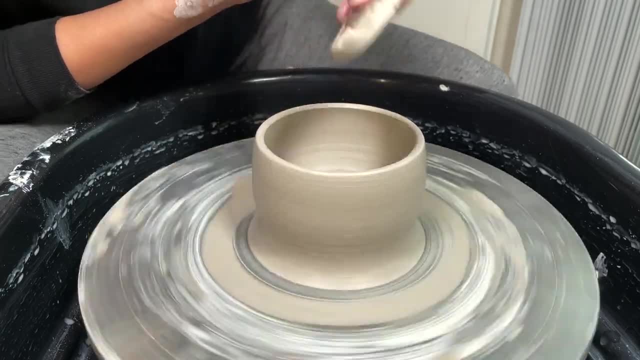 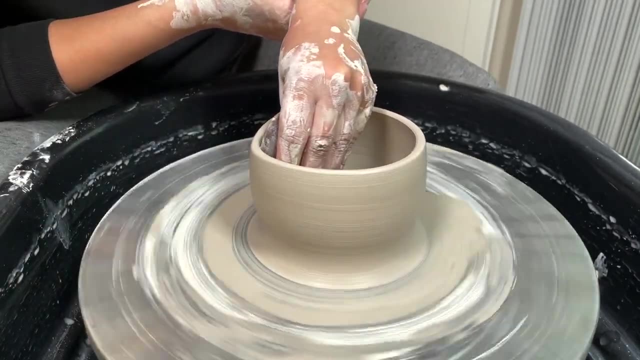 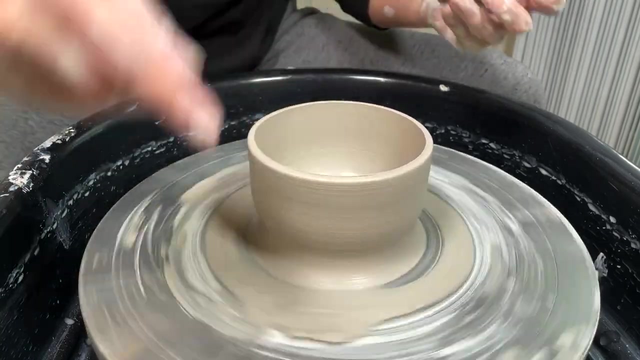 to shape my piece. our clay will come off during this step. we can wipe that right off and continue going and dip again and we can continue going over any areas. we want to adjust things we want to avoid. we really want to be careful that we don't have sitting water in. 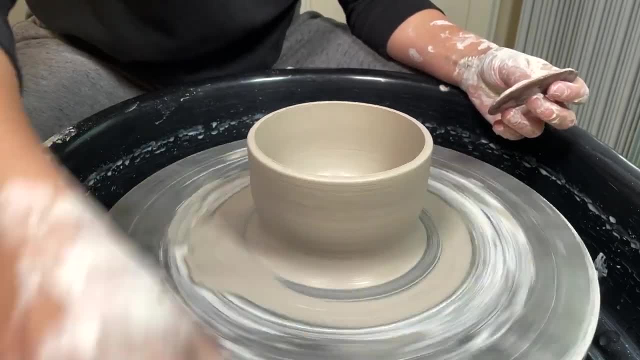 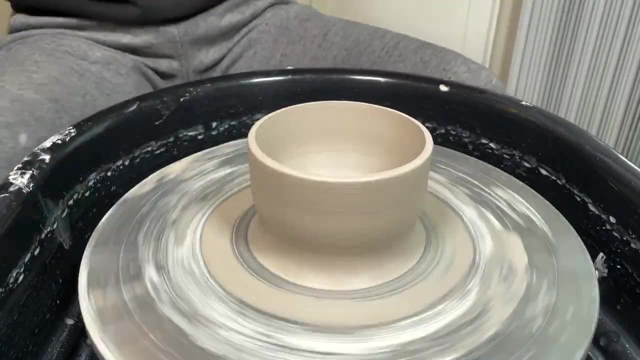 the base of our piece. that will sit and erode and lead to cracking. so we'll use our sponge to wipe any sitting water if that comes up. uh, and then you can go ahead and continue shaping until you're happy, i think for this piece i'll open it up a little more. 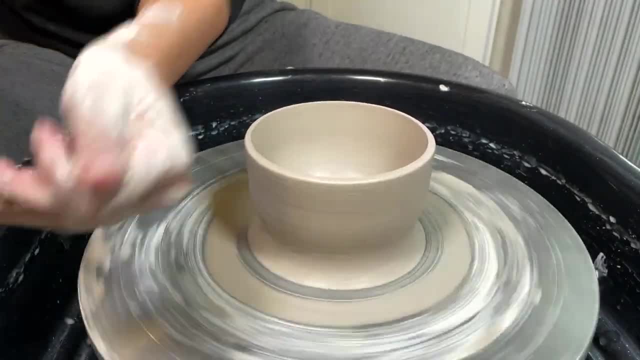 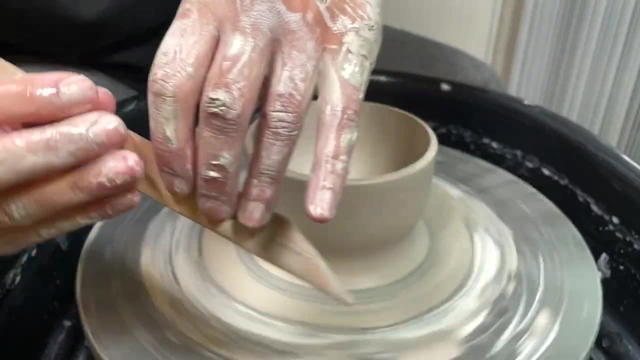 and then we're ready to go ahead and trim that foot using our wooden tool. so for this we have our blade side up, i'm holding it with my right hand and my left hand is on the top for support. i'm going to first find that angle. 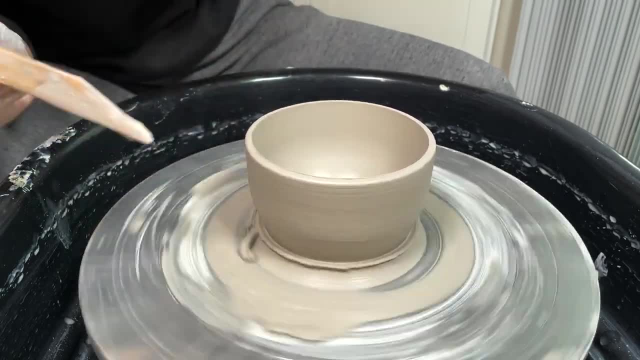 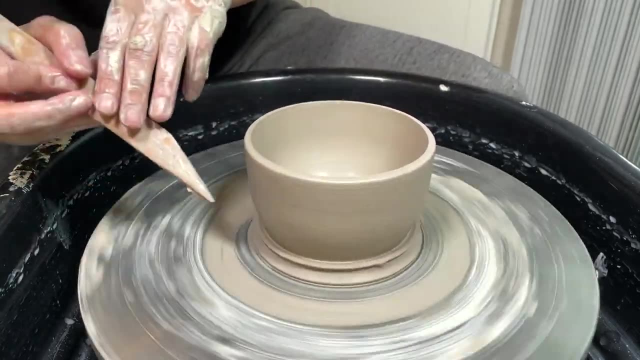 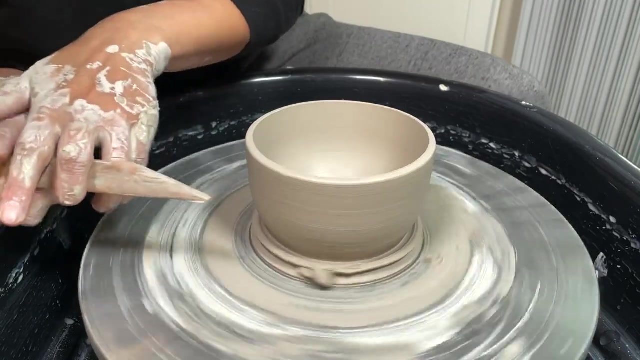 that my bowl has already and keep going. i want to be careful, um, not to start on the bottom and push in. that will push our clay up against our bowl. what we want to do is start high and cut that clay a little bit away, so we'll continue. um, if i go this way, we'd end up cutting all the way through, so we 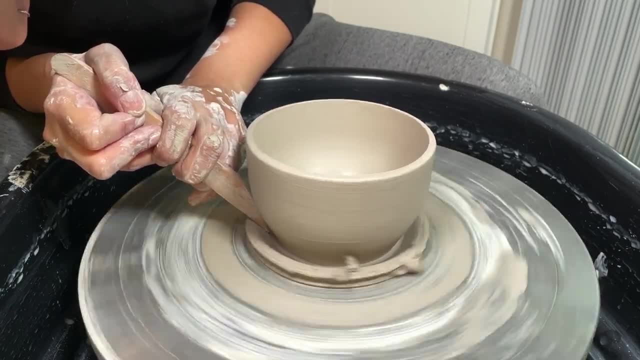 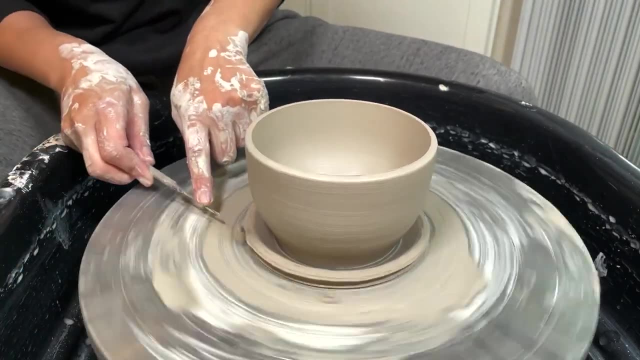 want to make sure that we're paying attention to the angle and cutting off just what we need. i'll continue until i see the wheel head and then with our needle tool, we can remove that clay, press down with one finger, slide in until we hit the side of the bowl. 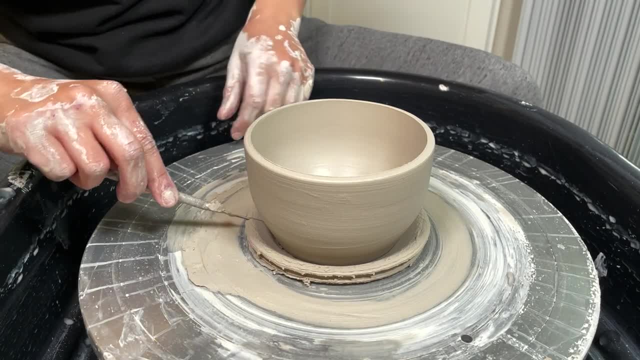 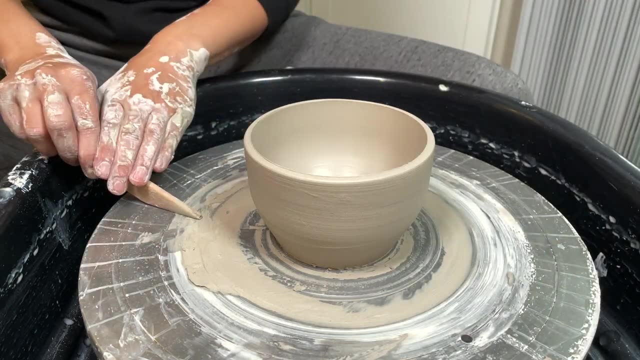 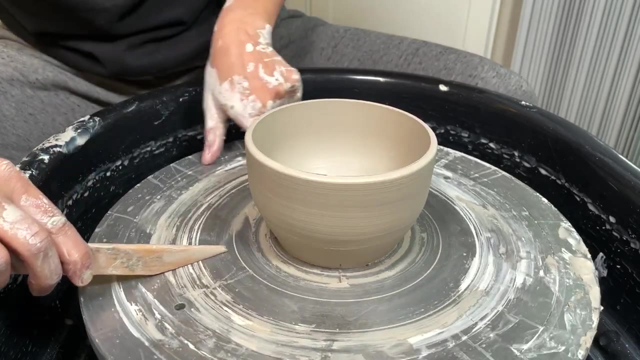 and then we can go ahead and press down with our heel to get the wheel off, cut through with your needle tool and pull that clay off. we'll go back to our wooden tool to clean up any of this clay. we want to angle our tool so the clay moves away from our wheel. 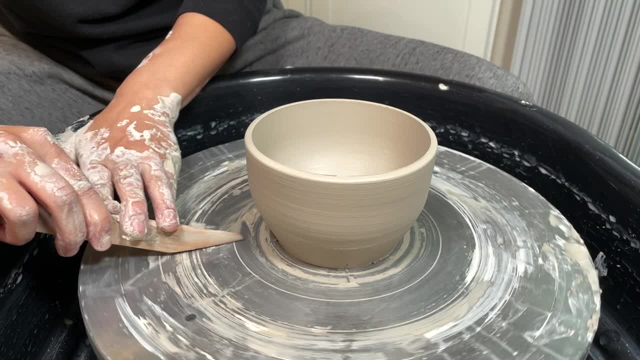 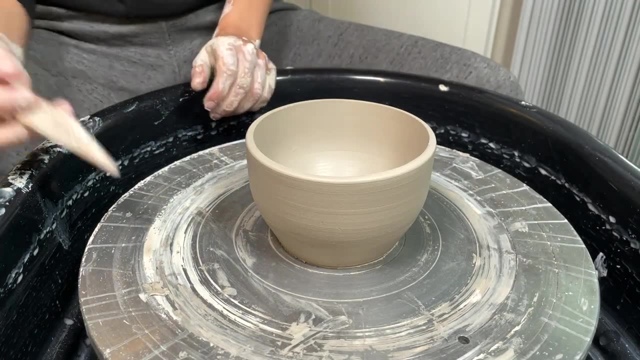 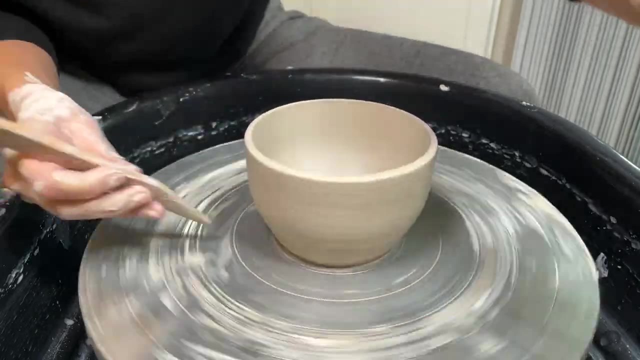 um from our bowl rather than benching up next to it and sticking. and in terms of touching up the foot and the sides, our wooden tool can do a lot. i can press this against the side to continue trimming, refining. i can go up the side to polish this out. 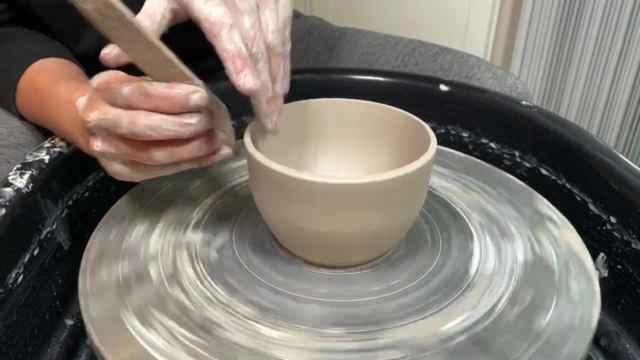 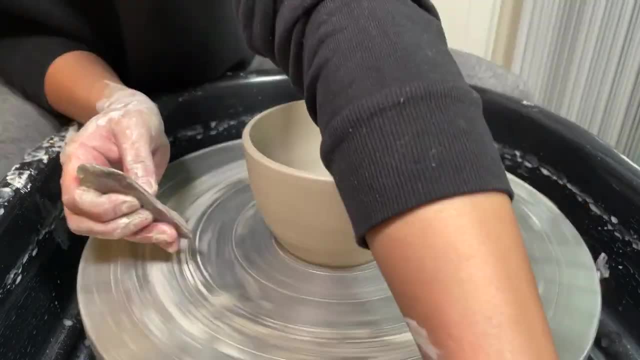 i can even apply pressure with my fingers or sponge. you can go in with your screed edge on your wooden tool as well to clean that up with your sponge. and this is just to if here there's any areas that the rib tool isn't quite reaching. 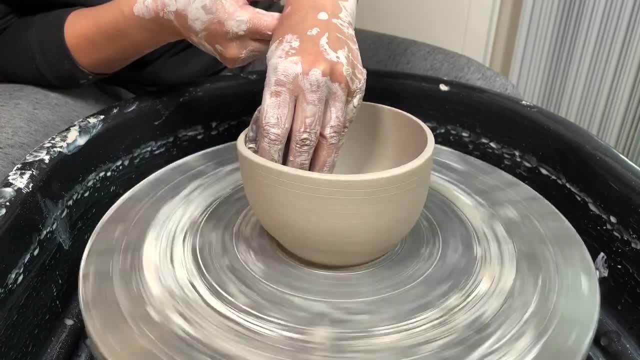 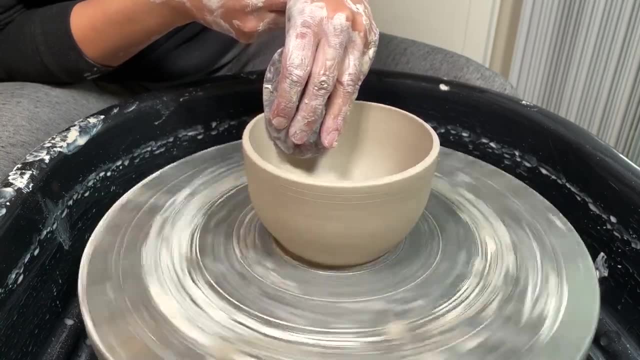 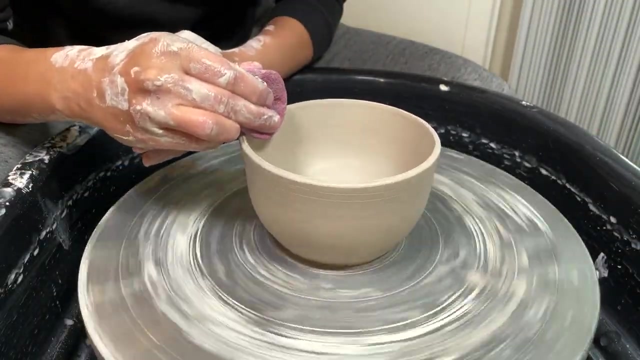 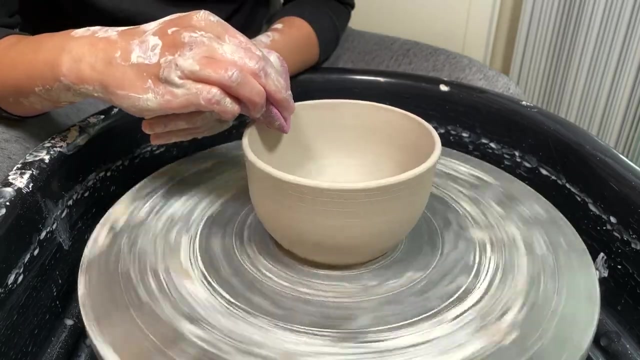 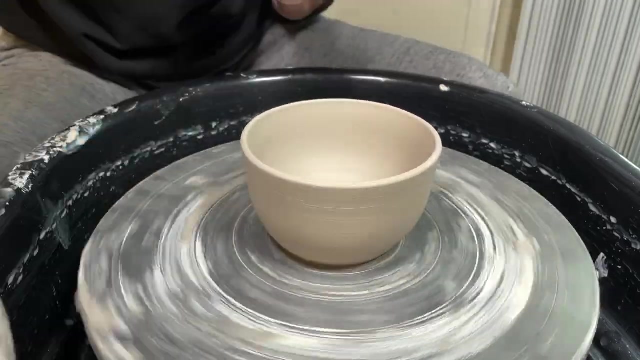 i might open this up a hair area. this is a you know good time to finalize any little last minute touches, kind of clean up our sides and the rim if you want to add any decorative elements. now would be the time some welcome to bed with care at home, when you or your home is going to be ways back. a lot of some things you can maybe keep intact somehow and have to bake and modernize sediment as well for something new. if you 먹을 at home with anger on a piece to see that egg grilled off the sides of theいき and you want a two by four, so be sure to get fire from your regular or poisoned tässä-mat 나는 부분이 to do the bake some dishes. 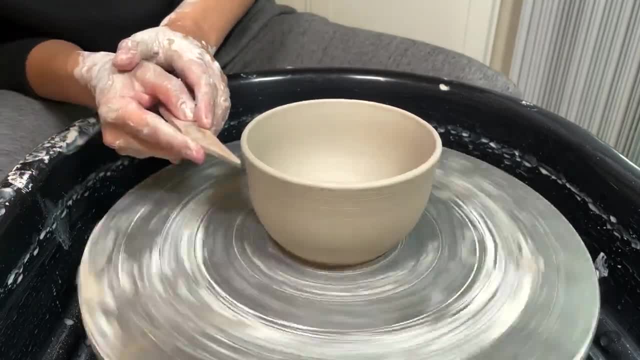 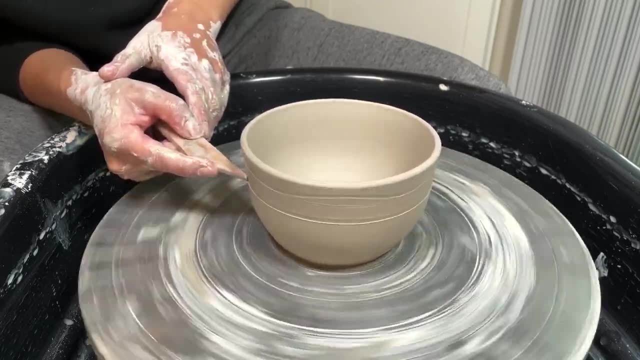 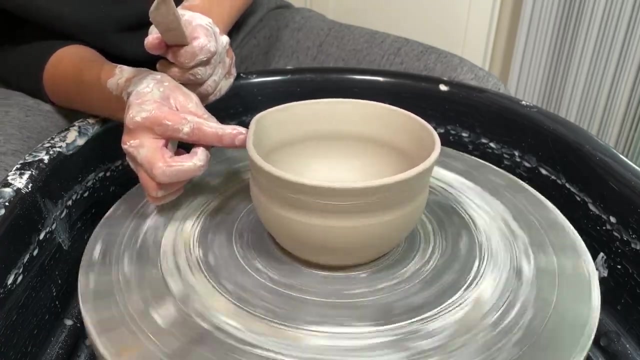 you can do with the tools you've already seen. You can use the- not the blade side, but the straight side- to do some decorative elements. You can use your fingertips even- And let's say you didn't want that and you wanted to remove it. 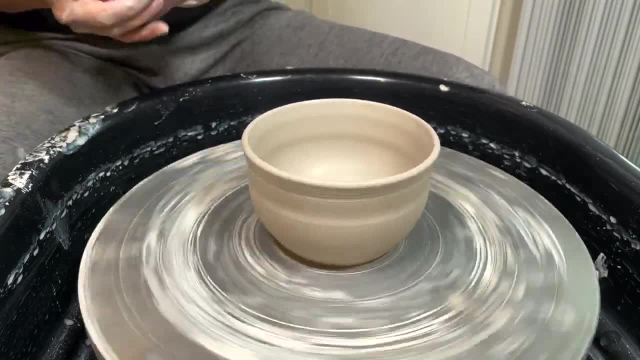 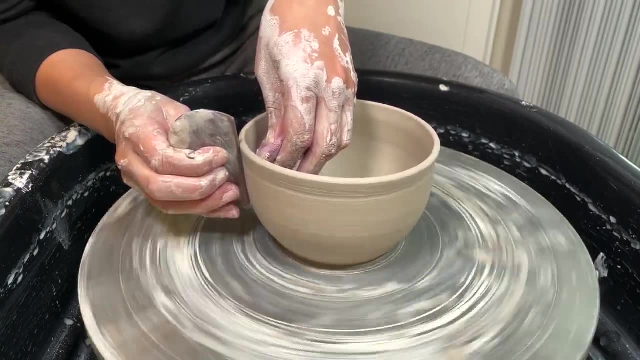 you can even go in with these tools and get it right back to where you were. So, using your rib on the outside, your sponge on the inside, you can get back to where you were. So there's a lot of options. 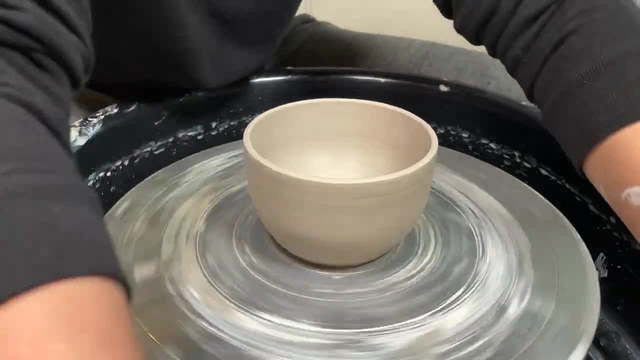 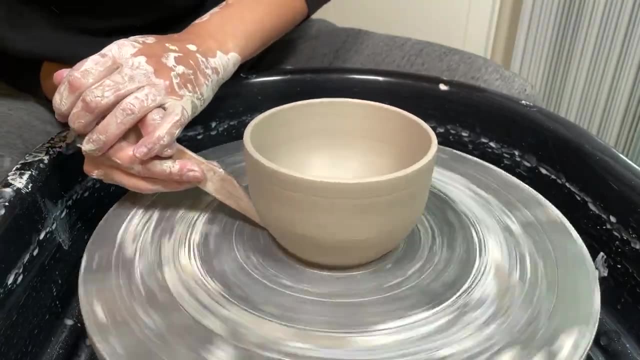 Whenever you're ready to go ahead and get your piece off, you can go ahead. and oh, you just wanna touch up the base real quick. That'll make trimming a little bit easier, And it's you know, before we get this off the wheel. 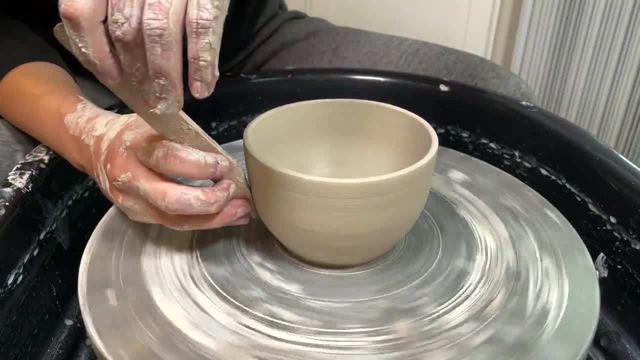 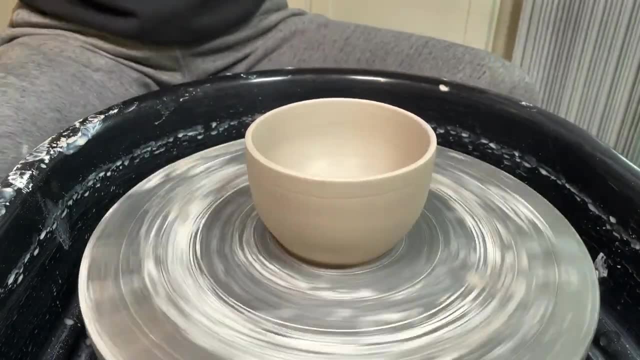 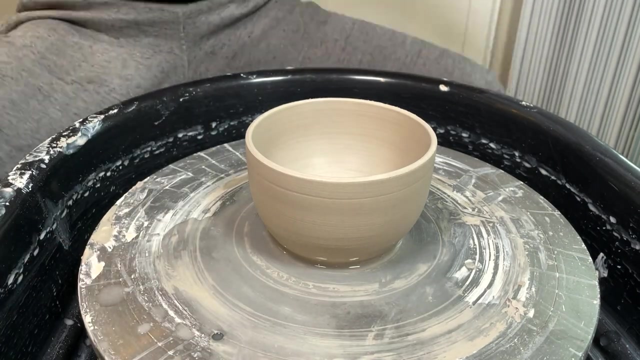 I'm gonna go ahead and get this off the wheel. You wanna get all this little stuff? All right. so we'll go ahead and get our wheel off, splash water on one side and get our wire tool nice and taut and go all the way through the base. 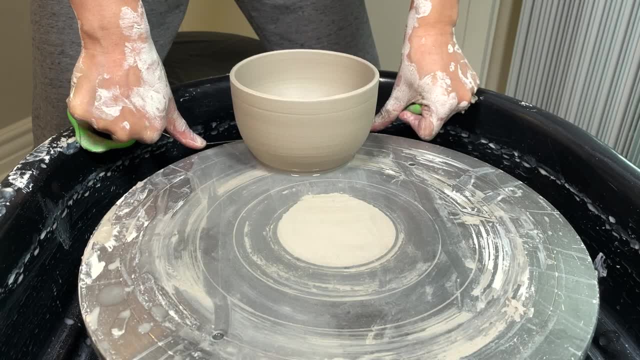 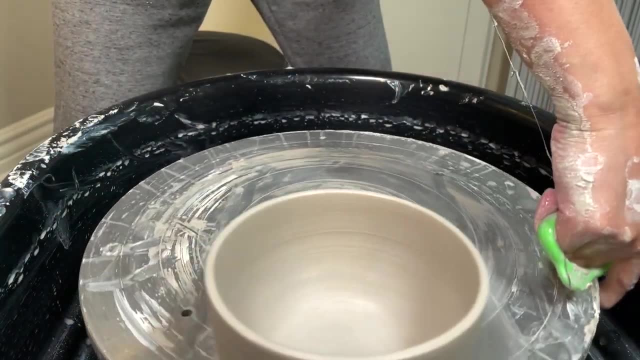 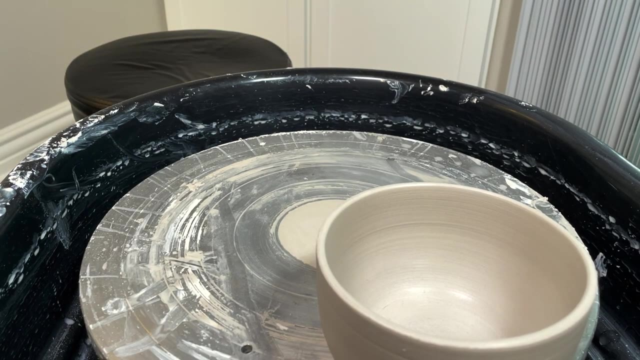 And we want to see movement And my wire tool. I'm keeping it down and going all the way to the side. I'm careful not to cut off any of the extra. I just want to go straight and down And then from here I can take my wear board.